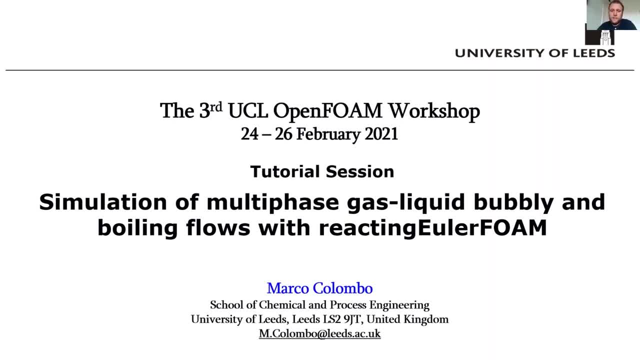 Perfect. So I'm very glad to be here to do this tutorial And, as mentioned, it will be focused on the simulation of multiphase gas-liquid bubbly flows and boiling flows using reacting Euler foam. I want to first try to give an introduction on reacting Euler foam and, in more general, on the multi-fluid model family, let's say, and then going on to two examples or two cases- one for a bubbly flow and the other one for a boiling flow- that I have also updated on the Dropbox repository. 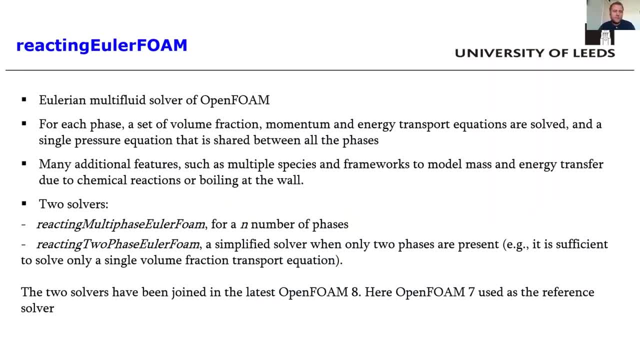 So, Okay, Okay, let's start. So the two cases will be based on the use of reacting Euler foam, which is essentially the Eulerian multi-fluid solver that is implemented in open foam, And what the solver does is solving a set of conservation equations for mass momentum and energy for each of the phases. 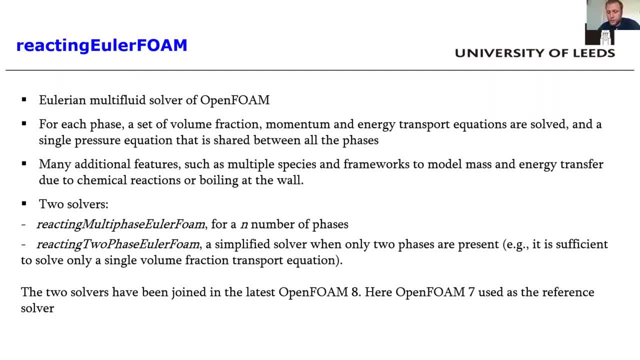 And a single pressure equation that is shared between all these phases. Now the model is essentially the solver, is the reference for multi-fluid modeling in the open foam and has many additional features. There are frameworks to implement mass transfer, to implement heat transfer, different species in a phase. 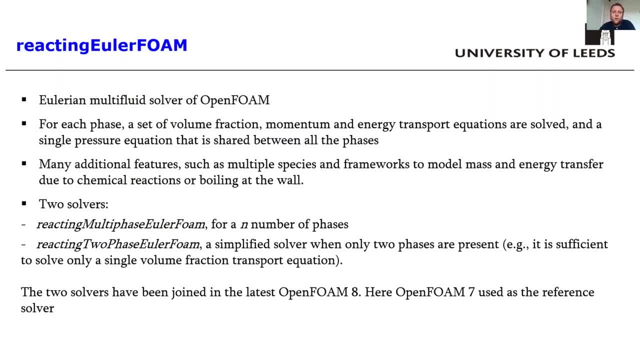 So it can be extended to cover many phenomena in multiphase So such as boiling, as I will give an example later on. There are, or there were, two solvers. One is reacting multiphase Euler foam for an n number of phases which I will be using. 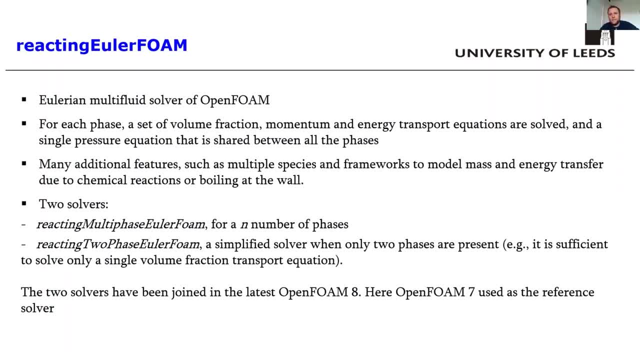 And reacting two-phase Euler foam, which is more or less a simplified version of reacting multiphase Euler foam, because it's implemented only for two phases. So in this case, for example, it is sufficient to solve for one phase, So for one equation for the volume fraction, because the other one is automatically given. 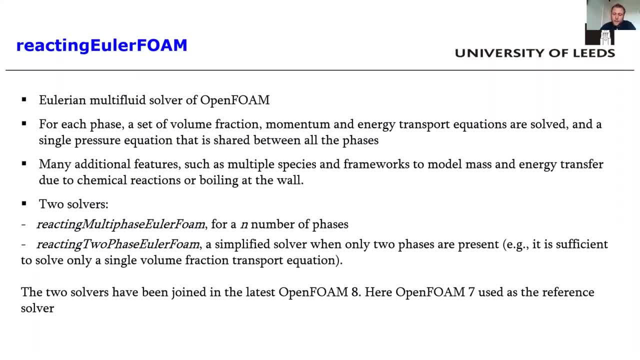 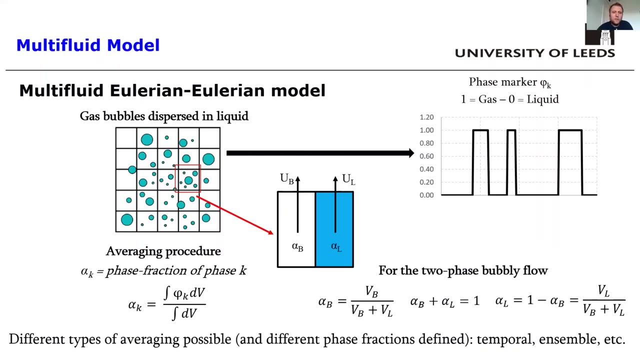 This was until version seven. Now, in open form, eight, the two solvers have been joined into one single solver. OK, so a few words about multi-fluid modeling. and what is multi-fluid modeling about? So, if we consider, I don't know. 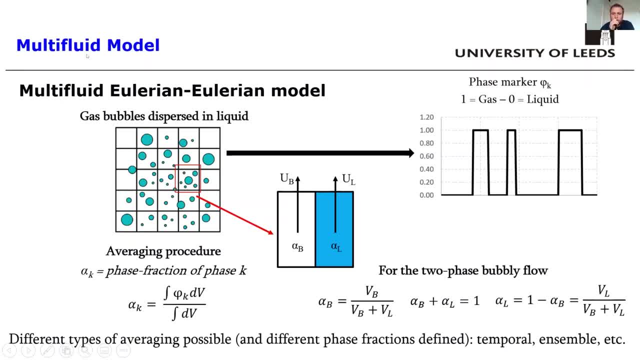 I hope you can see my, my mouse moving on the on the screen. If you consider gas bubbles dispersed in a liquid such in this case. Now, if you imagine to have a phase marker function, which is which assumes the value one in gas and zero in liquid, 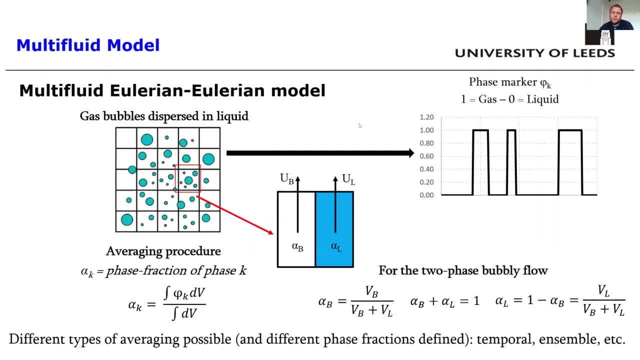 If you do, if you fix in a, in a, in a point or in time, or their point in time, and go through time, that, Or also if you go through In space, that function will go from zero to one If there is gas and or or liquid presence. so no other conditions are possible because there are well-defined bubbles present. 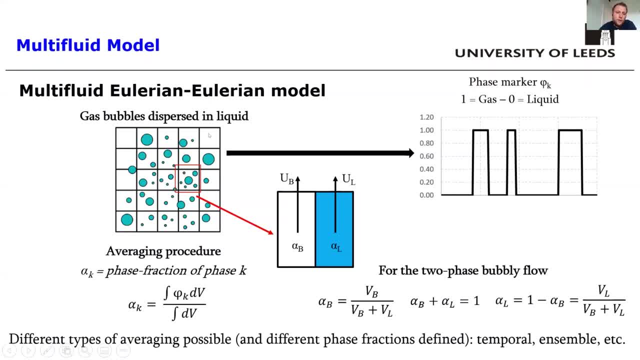 So what multi-fluid modeling does is take an average of these of these situations. So if we imagine to do an average over one of those, a cell, and we integrate that function that goes through Zero to one in that cell, what we end up with is more or less the volume that is occupied by the gas phase in that, in that cell. 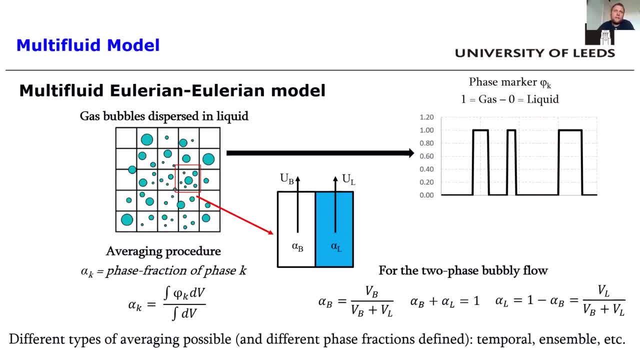 Now there are different formulation of the multi-fluid models derived, which different methods of everything based on time averaging, space averaging or ensemble averaging- but the basis of the equation are the same. So what happens if we average this domain and other than that phase marker, we average also velocity. 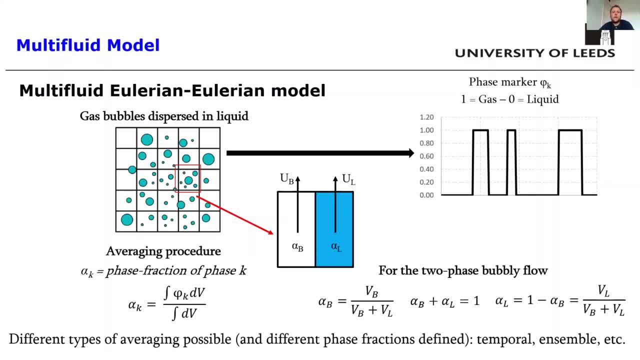 We average also density, We essentially end up with these Situation here: We don't have any more bubbles in that, in that space, but we end up having simply Some volume of gas and some volume of liquid in the same cells. Each one having is his own velocity. 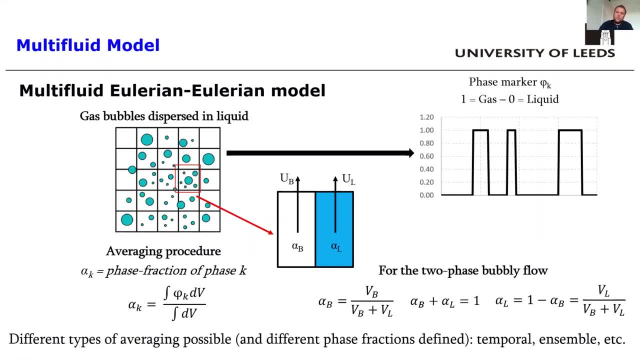 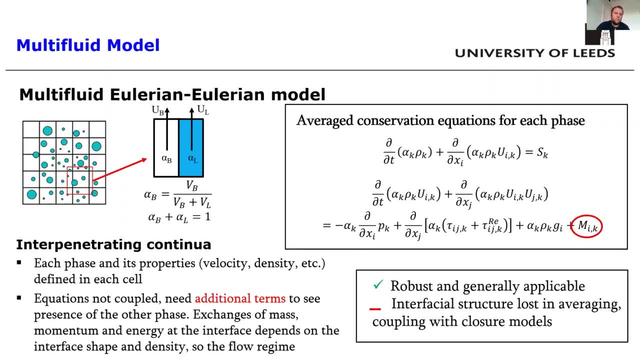 So, So, So, essentially, we derive what is called the concept of interpenetrating continuum. So we don't have single well-defined bubbles anymore, but we have some gas, some liquid, and each phase becomes present everywhere in the space with its own property, density and velocity. 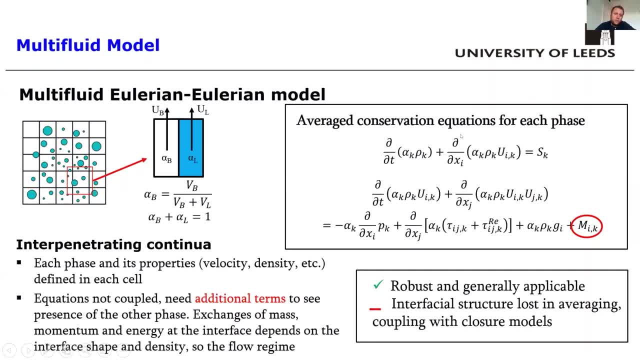 We are able to derive, as you can see here in the box, two different sets of conservation equation: Mass, Mass, So one for the element and then One for thegencis. So for the element and energy, one for the. 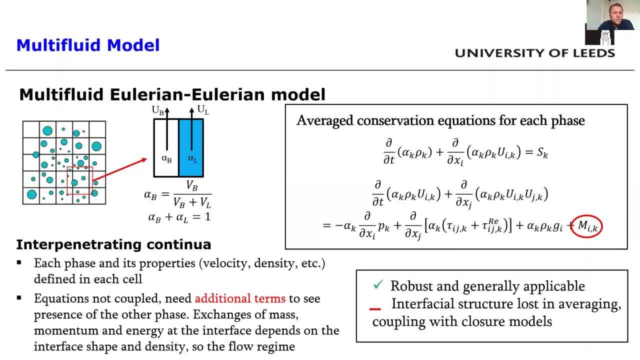 And one for the liquid, And in this way, we today a model that is quite robust and generally applicable. with that I mean that, Given that you don't need the true It's single bubble in the field, Now the model is quite 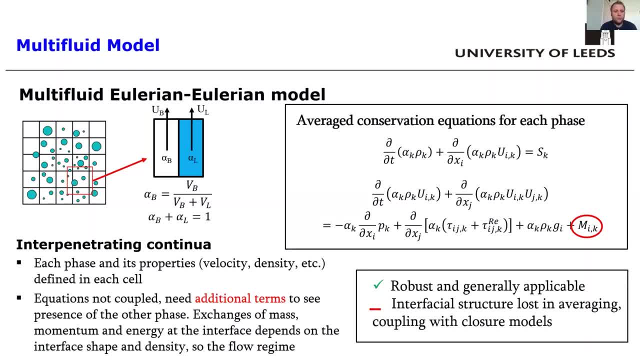 Easy applicable to very large, complex domain Where you have a very large number of bubbles Domaine that are quite difficult to see be locked with CFD if you need to resolve all the single bubble shapes But at the same time the complexity. 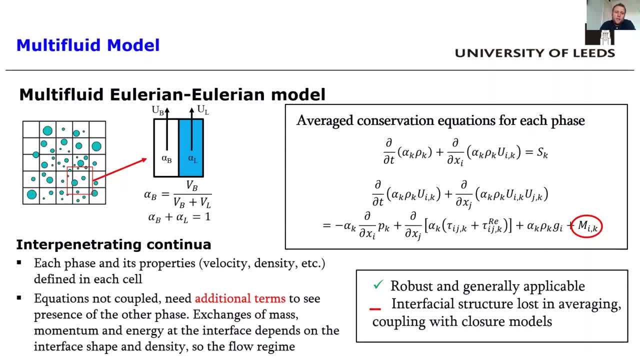 that is introduced. by doing this averaging is that we lose the interface. We don't have the interface anymore. We simply have some gases, some liquid that flows in that cell and they don't see each other unless we close the system of equation with additional terms. 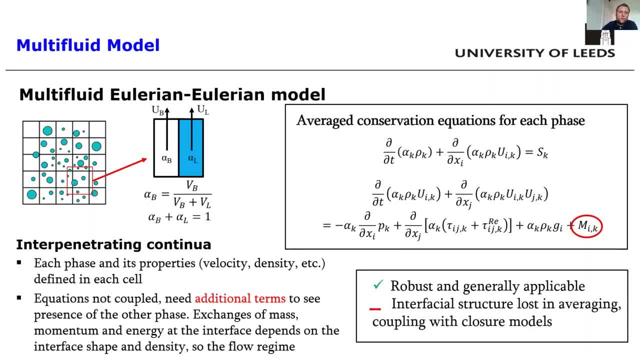 that needs to be modeled, of course, because we don't. we don't know anymore about the surface of the bubble, So we need additional modeling to represent the interaction of the interface between these two phases and all the exchanges of mass momentum and energy at that interface. 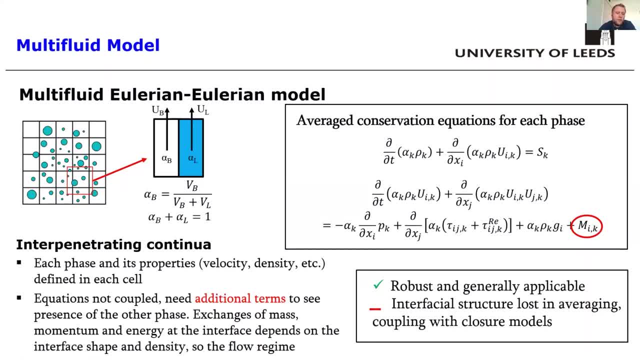 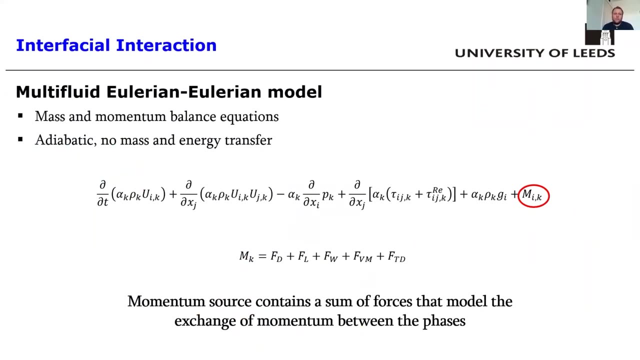 And of course those terms are function of the inter-save shape that we don't know. So for small bubbles, some the physics is different that for larger bubble and is again different for, for example, stratified flow of some gas and some liquid. So to go into a bit more details, if we focused 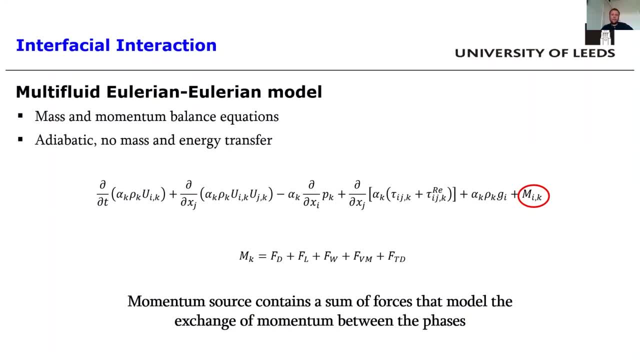 on a system, an adiabatic system. so we don't have mass transfer and we have only a mass and momentum balance, equations, and you can see the momentum balance there. So that equation will be- will be solved, one for each phase, as I said. but what couples? 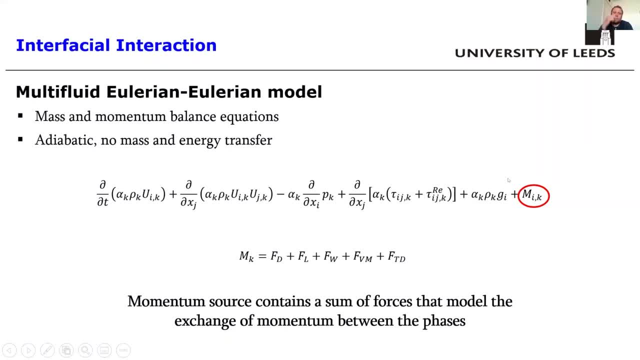 the two. the two phase is is these terms: m, which is in the momentum equation, is the sum of the forces that act between the phase and is needed in that model to model the interaction between between those two phases And generally the force is that that are included in these. 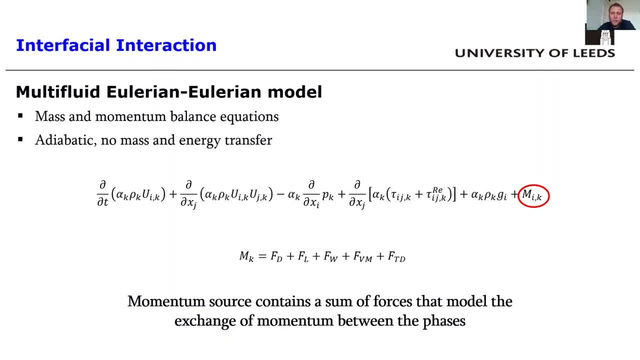 two phases to make this later with that, some form of experiment, because otherwise you won't be able to jumped an X, But nonetheless still a better way to draw that real car to. in those terms, um are a drag force, a lift force, uh, a wall force, virtual mass and turbulent. 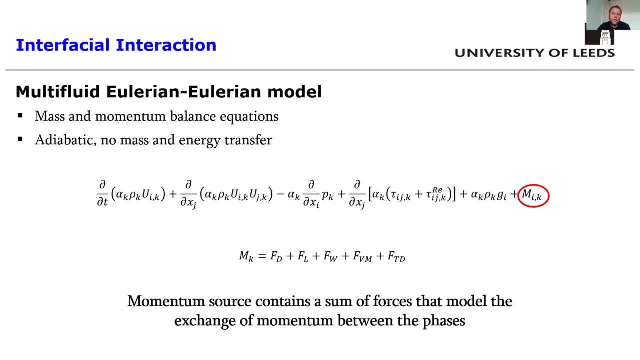 spatial force, so five forces, to model uh the interaction between uh the gas bubbles and and the liquid phase. and without including these, these forces and proper modeling of these forces, the two phases uh won't see, won't see each other, essentially, except for uh the geometric constraint, so that uh, given that drag, two phases, one phase cannot occupy the, the entire volume there. 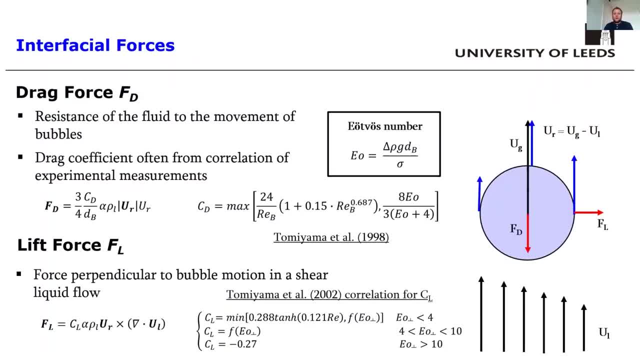 so, uh, let's, let's try to to give an example on of two of these forces, of how this, this modeling, works. so, if we have a bubble here, that is, that is, imagine that is rising in the, in a liquid, in the vertical direction. so the bubble, because of words, will be faster than the liquid. 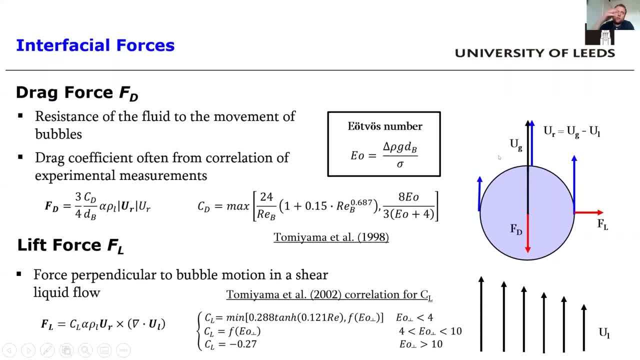 which means that there will be a flow, a recirculation flow, of the liquid around this bubble and this exerts a force on that bubble that if we use, for example, a volume of fluid model, we resolve in the computation. in this case, instead, we need to model that, and that is modeled with. 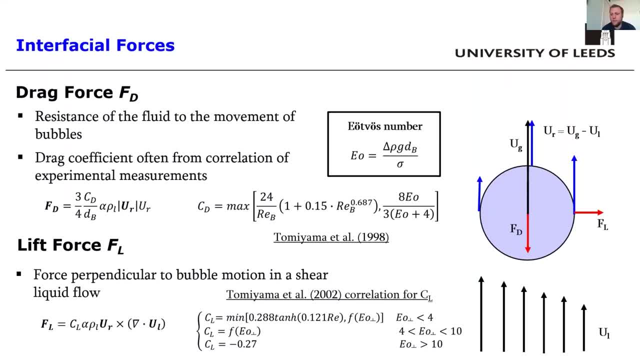 the drag force, which essentially models the resistance from the fluid to the movement of the bubbles and enables calculating the right rising velocity of that bubble. you see the um in the in the, the equation for the drag force and how that is modeled, in particular the drag coefficient is uh, with an empirical, an empirical correlation. 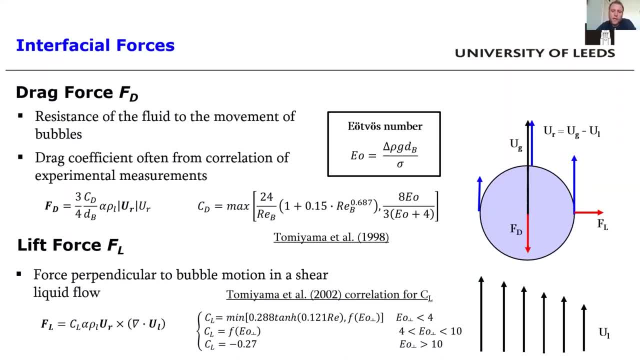 function of the bible or uh bubble reynolds number and or the autobus number. there are different kinds of correlation and many are. are the options also available in react singular form at the same time? uh, imagine that. okay, if, if there is a shear flow and not a? 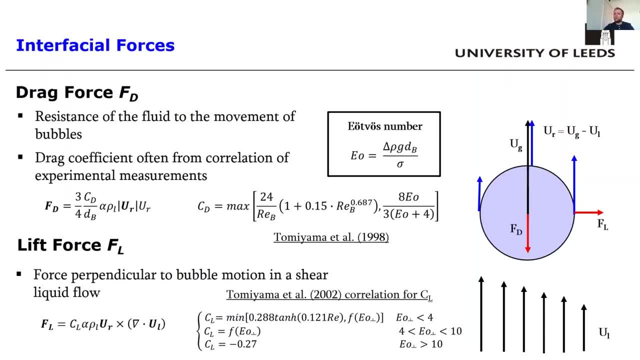 for example, a creation liquid, but there is a flow also of the liquid and you have a gradient in the liquid velocity. that means that the recirculation is not symmetric around the bubble surface and this will generate will generate a force that is perpendicular to the main bubble motion and 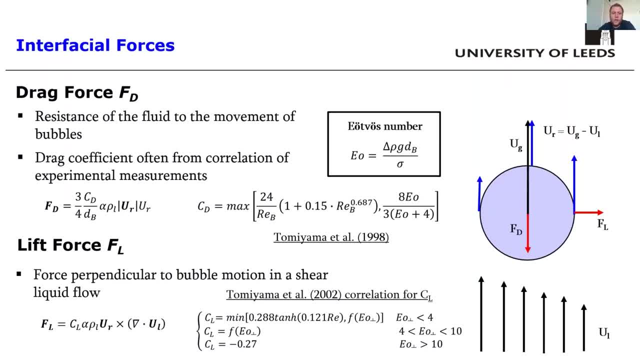 this is known as the rt and this is what we normally call the lift force. and we need in this, in this model, an additional sub model to model the action of this lift force- that that you see here- and another correlation to um to model the lift coefficient. one of the most used is the tomyama correlation for that lift. 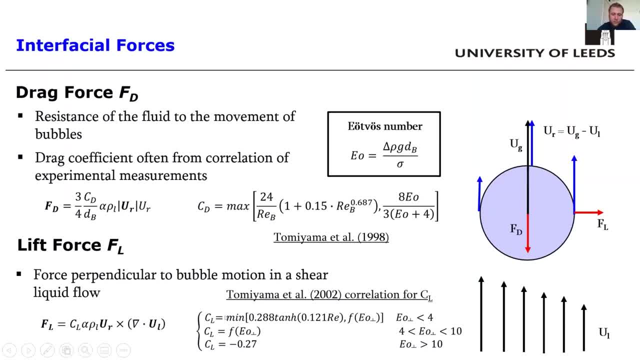 force and the things to say about this correlation and about the lift force for bubbles in general, and that this goes from point to point. this goes from positive for spherical bubble and to negative for very large bubble that are, that are deformed, that therefore are so small bubbles are pushed, in this case, to the right. 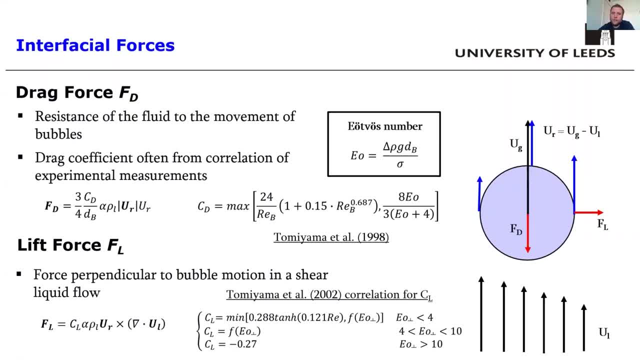 towards the direction of larger relative velocity and larger bubble will be pushed to the left towards the region of lower relative velocity. And I will speak also about the other forces later on in the tutorial when I will see how to activate those forces in the settings of the solver. 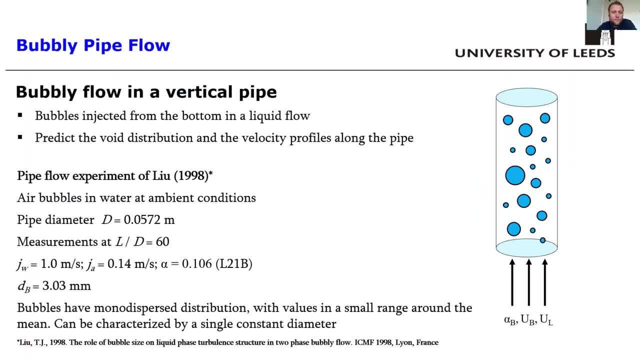 So this was a try to give a quick overview on the basis of this kind of model, and now I will move on to the first tutorial, which is the simulation of a bubbly flow in a vertical pipe. So we have a liquid vertical flow in a pipe with velocity coming in from. 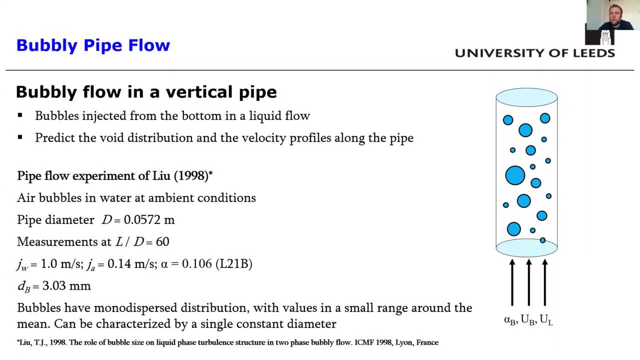 from the inlet section and at the inland section that are also bubbles that are injected in the flow, And what we want to do is being able to predict how these bubbles distribute in the pipe and also how they affect the fluid flow. So I've used as a reference the pipe flow, using the 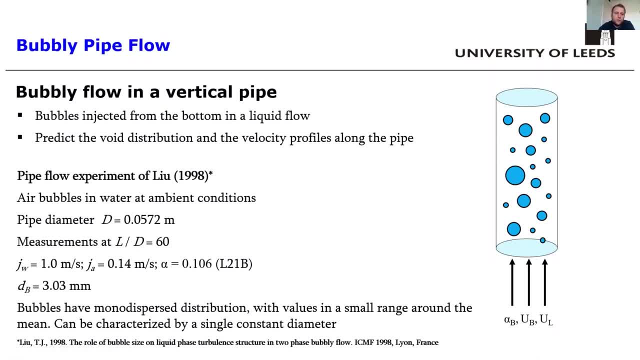 experiment of Liu, so that we can also do a little bit of comparison against some experimental data. It was an experiment done with air bubbles in water in ambient conditions, sorry, And the pipe diameter is a bit more than five centimeters and measured at a distance of about. 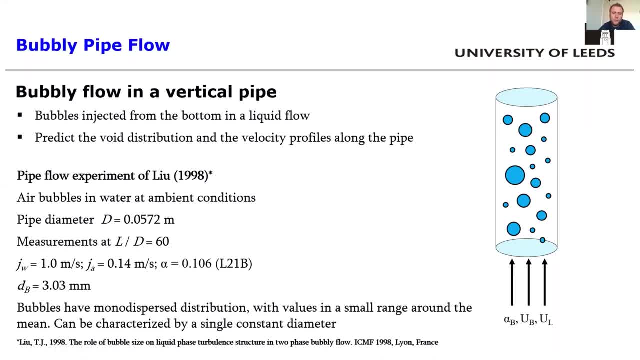 50 kilometers per second. So the measurements were taken at 60 pipe diameter from the, from the inlet section. So what? what do we know? We know the superficial velocity, which are essentially derived from from the mass flow rate of the two phases. We know the volume fraction of the gas. 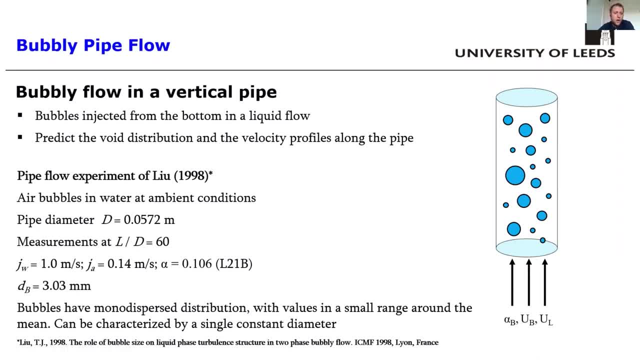 and we also know the average bubble diameter of the bubbles. Now here are important things to mention. This case and I you, I've used this case because bubbles have what is called a monodisperse bubble distribution, Now normally in a in a bubbly flow. 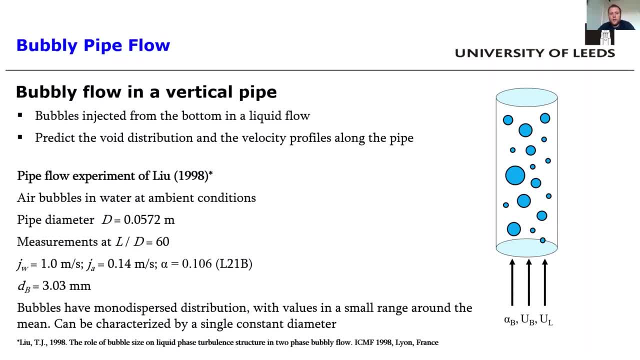 bubbles have different size and which means that their interaction with the fluid changes as a function of the size. If you see here drag force and lift force: in all these models there is the bubble diameter, So drag and all the forces changes, going from a small bubble to a large bubble and 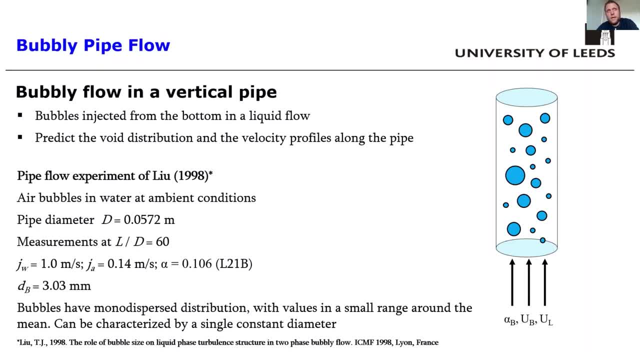 the bubble change their behavior. For this case, bubbles have almost all the same size. That means we don't really need to characterize the full spectrum of the bubble diameter, but we can represent that population with a single constant bubble diameter and we we will see later on what this means. 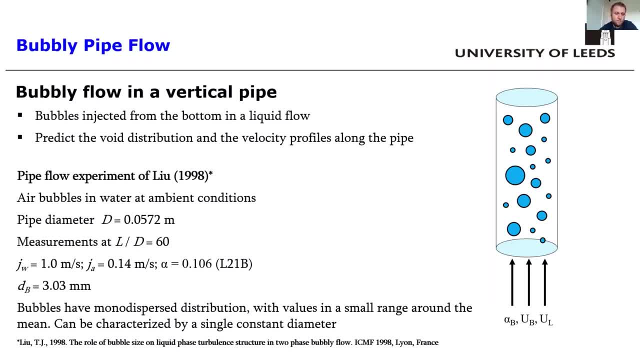 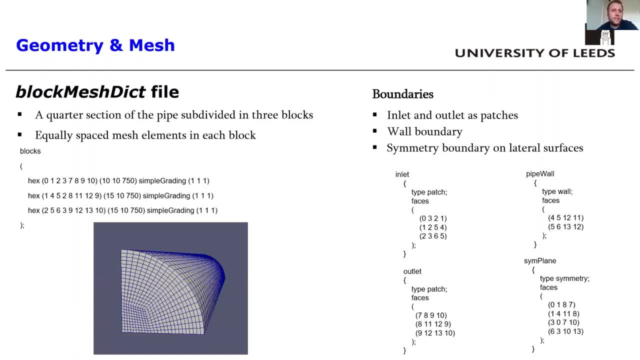 when that's not possible for the boiling flow case. Okay, so let's start with with the starting up of the case from the geometry and the mesh. The geometry and the mesh were done using block mesh and what I've done is essentially create a one-quarter section of that. 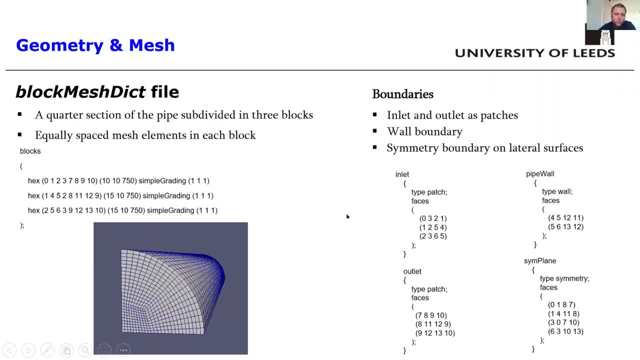 pipe and to create, to be able to do a good structure mesh. I've divided that pipe in three blocks: One small in the center and two portion to round the portion on the outside. Now this, the internal part, is 40% of the total radius. 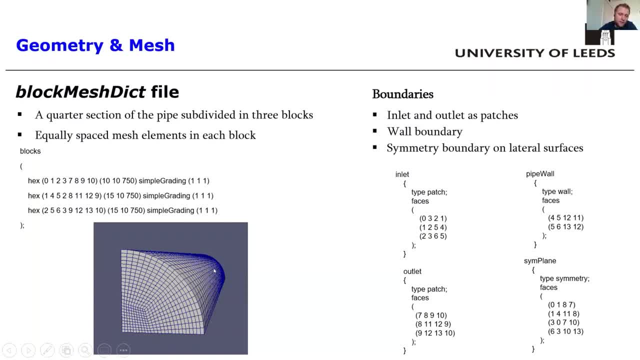 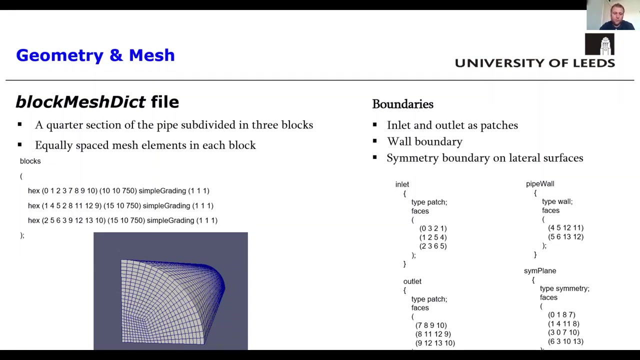 but that's actually. that's not a fixed value. it can be changed and different configurations can be used. You see the definition of the blocks here on the left and the mesh element used to mesh the pipe. I can. what I plan to do now is try to switch a bit between the presentation and the file. 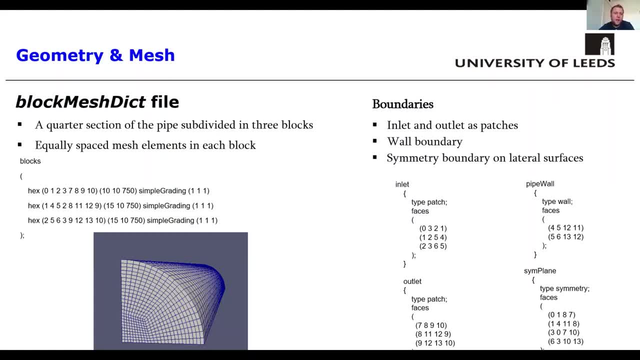 and so if we have a look at the block mesh, you see the definition of the vertices there. I've put the main features on the slide, but the three blocks defined with the mesh, oh yeah, what I was going to say is that I've used equally spaced mesh element because I'm using a high 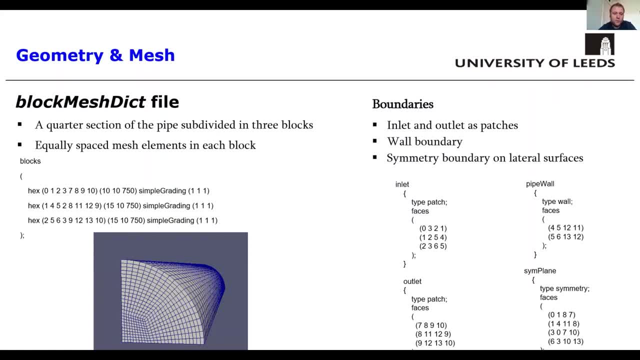 Reynolds wall treatment and it's fine to use equally spaced elements in this case. Of course, you have to define curved edges on the wall surface of the pipe and the other thing to say is that the boundary definition we have the wall uninerted outlet patch and also the two lateral. 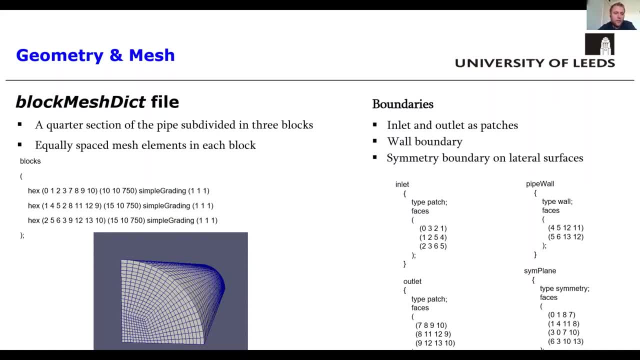 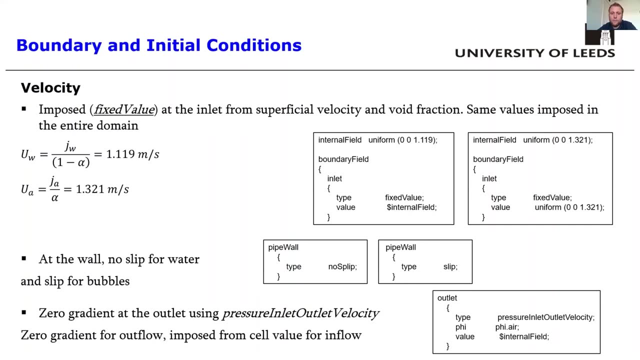 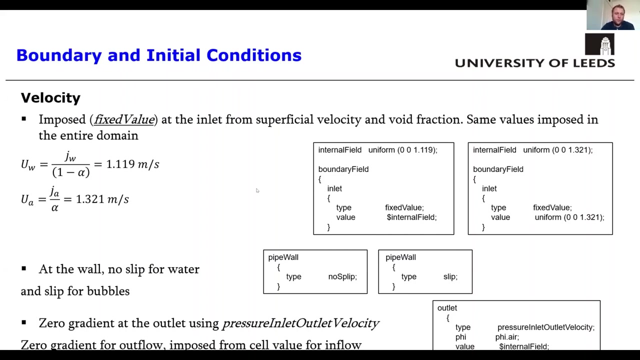 surfaces are defined as symmetry, and they are a symmetry. boundary condition is imposed for all the variables and all the relevant variables. Now, instead for boundary and initial condition, let's go back again to the case. of course, we have the typical structure of an open form case with the zero folder constant system. you see. 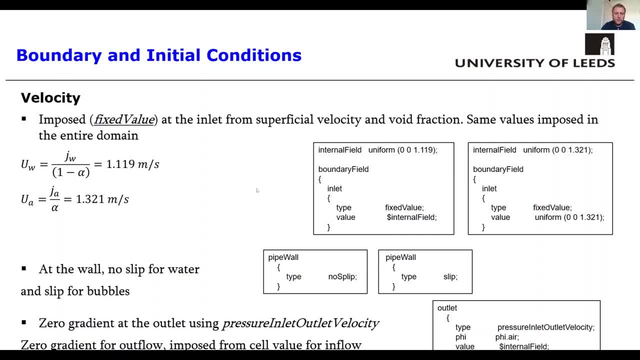 and the results are also there in this case. So here you have all the variables at the beginning of the simulation that you need to set up. We still have temperature there because the model solves also for energy. it's essentially an idea about in case temperature remains constant across the simulation. 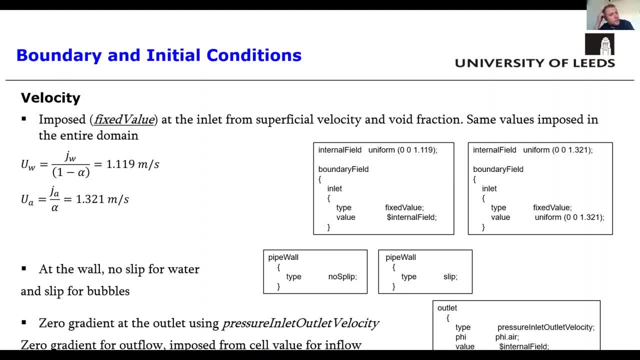 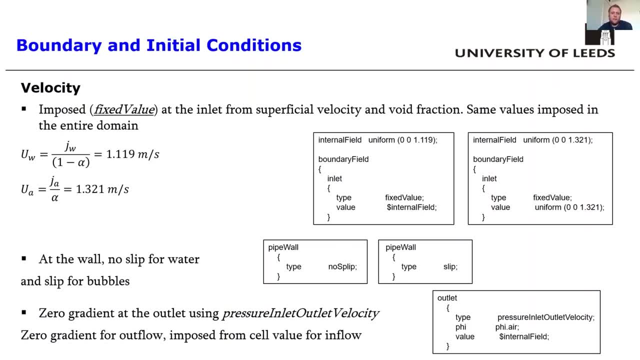 So let's go back to the presentation and see the main, most important things to set up between boundary and the initial condition. So the velocity is imposed with a fixed value at the inlet and the velocity is calculated from the superficial velocity that we know and the volume. 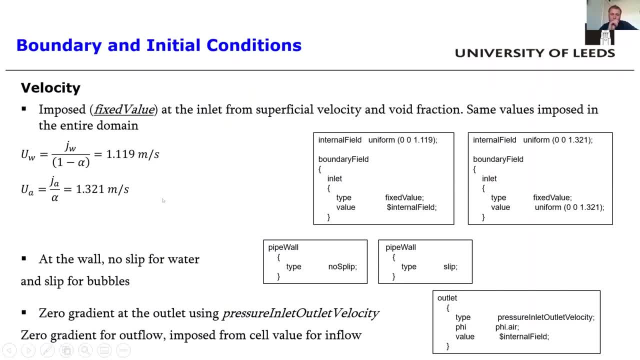 fraction of the gas, and you see here the results of the calculation and the value of of the velocity. Those values are considered uniform on the inlet section and also uniform in the domain at the beginning of the simulation and instead at the wall we have a no-slip condition for the pipe. 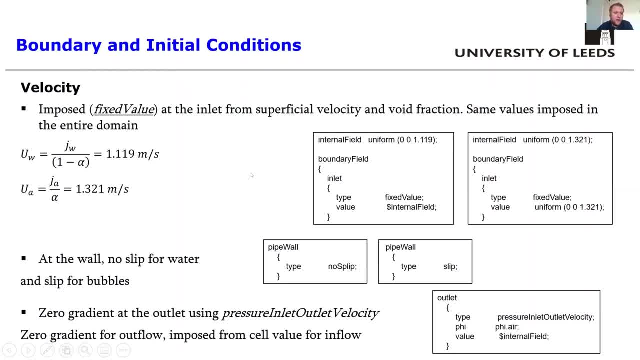 and instead a slip condition for the air. Instead, at the outlet, we imposed at zero gradient condition. but instead of imposing the normal zero gradient condition we use this pressure inlet outlet velocity boundary condition, which essentially says that if there is outflow, there is a zero gradient condition, if, during there is inflow, 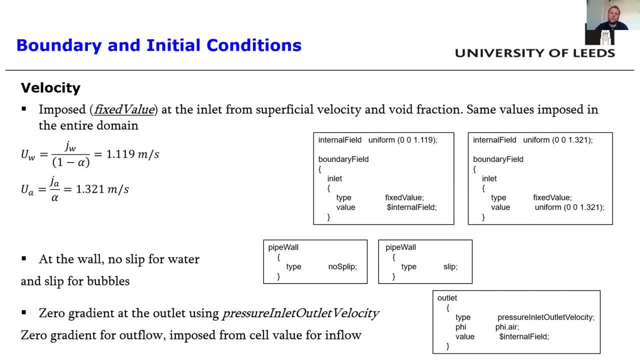 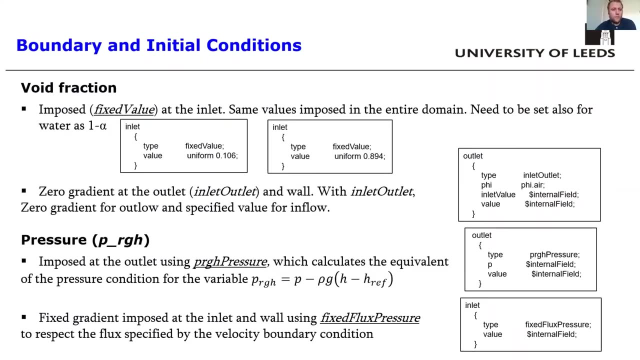 the value of the velocity is imposed from the value in the nearest cell and you also. you can see that the flux is set up to use to evaluate if there is inflow or outflow For the void fraction. we also used, again, a fixed value at the inlet section of the pipe. 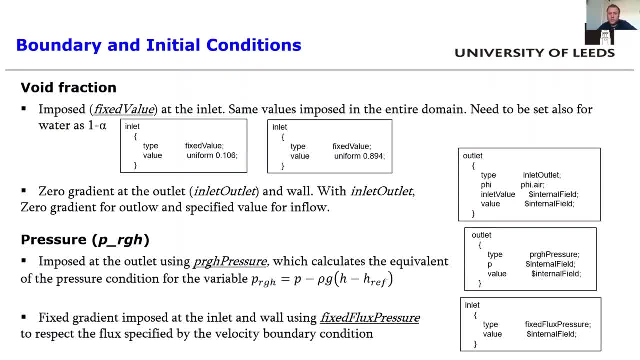 equal to 0.106, which is the value we know from experiment. Of course, we need to fix also the volume fraction of the liquid, and this will be one minus the volume fraction of the gas, Which is named alpha in all this, this presentation. 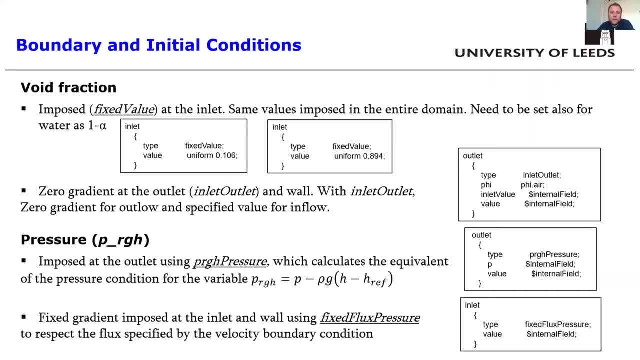 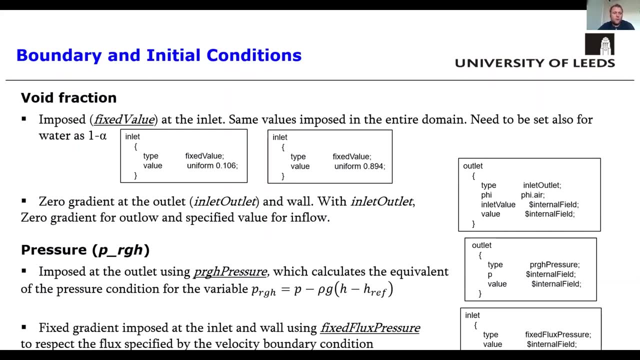 These values are you considered uniform at the inlet and also the entire domain? as an initial condition? There is a zero gradient condition at the wall. maybe I will show the file. So we have the fixed value at the inlet instead at the output We use this inlet outlet boundary condition. 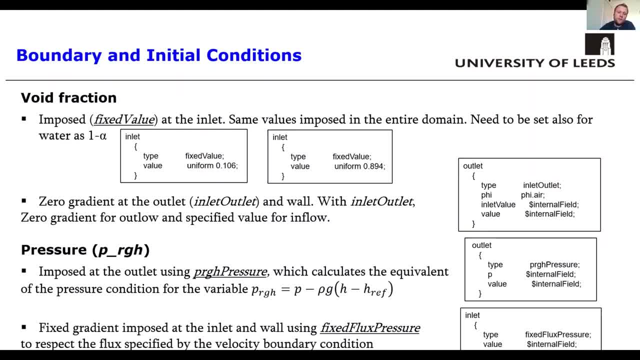 which is the same as before for the velocity. if there is outflow, it consider that a zero gradient condition. if there is inflow, from that condition the value of the void fraction instead becomes a fixed value, which is again fixed, equal to the internal field. Zero gradient at the pipe, and you see there the symmetry boundary condition, that is. 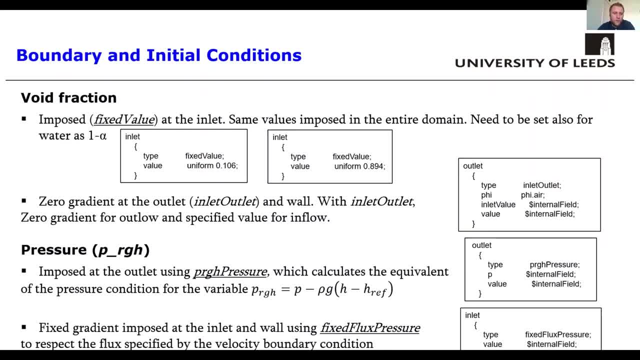 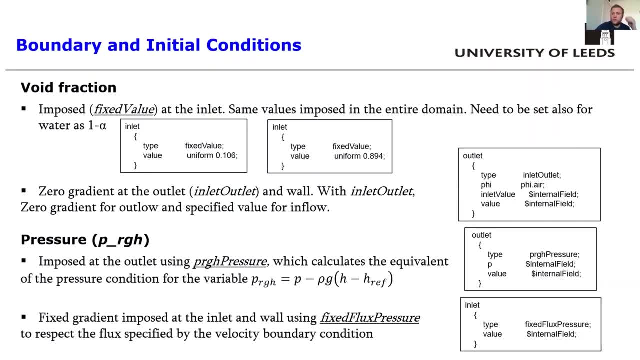 imposed on all variables. Instead, for the pressure, we used a fixed pressure condition at the outlet and using the PRGH pressure condition, because the model solves, the solver solves for this modified value of the pressure and this condition essentially calculates the equivalent for PRGH of a fixed pressure boundary condition. 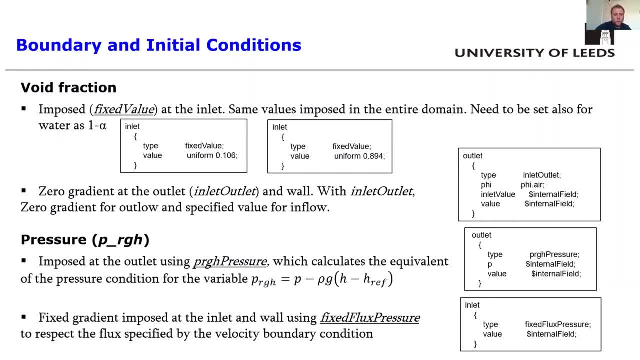 And the inlet and the in at the wall. we have a fixed gradient instead of a zero gradient, and that fixed gradient is imposed using the fixed flux pressure boundary condition, which means the gradient is fixed at a value that allows to respect the velocity imposed by the velocity. 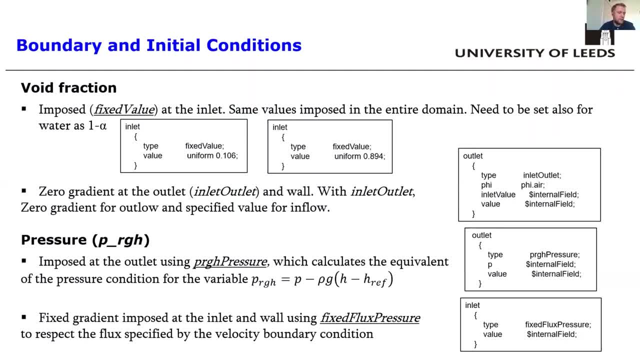 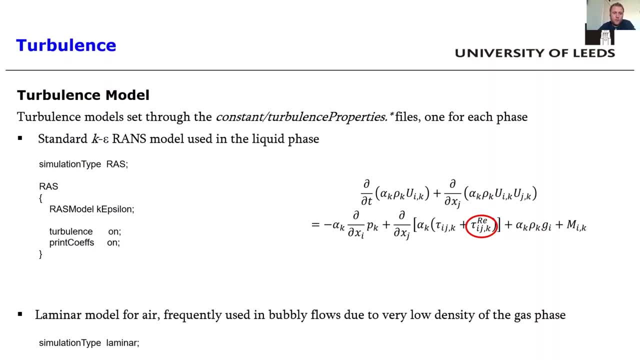 boundary condition on the same, of course, location. Okay, and this is almost well not everything. there is something later on a little bit more to say, but the most important features of the boundary condition for velocity, pressure and volume fraction. If we go back to our momentum balance equation, we have the m terms that I 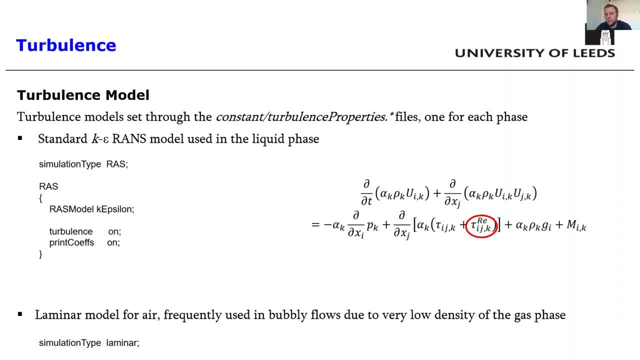 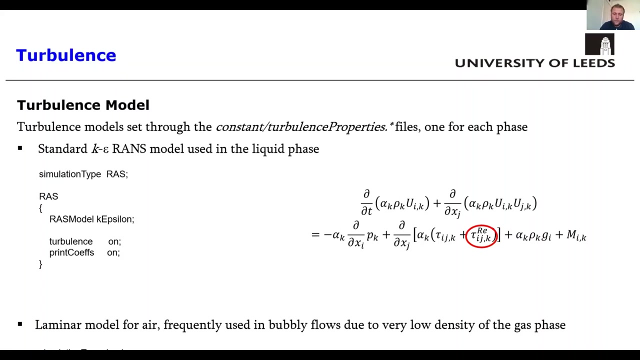 mentioned, but we also have an additional terms to solve, which is the turbulent, which is related, related to the effect of the turbulence, and so we need to couple to our model also a turbulence model and the models, the turbulence model are declared in the constant, in the constant folder, and for these models we need to define. 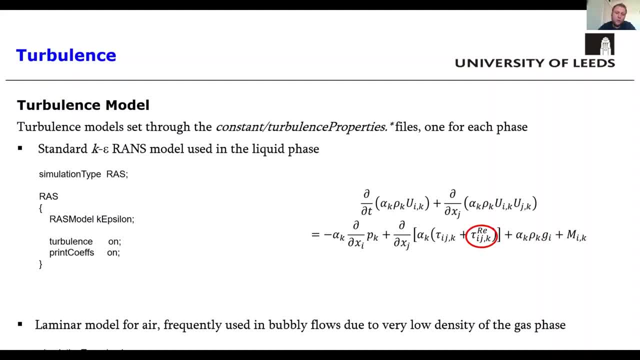 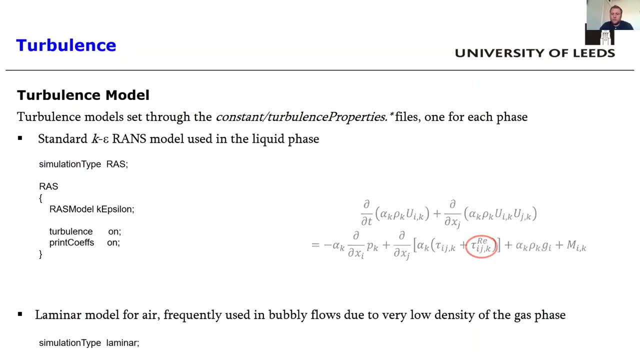 you see, there we have turbulence properties for water and air, so we will need to define a turbulence model for the water or the air, and different options are possible. In this case we use a general K epsilon model for the liquid phase. so, based on the eddy viscosity assumption and 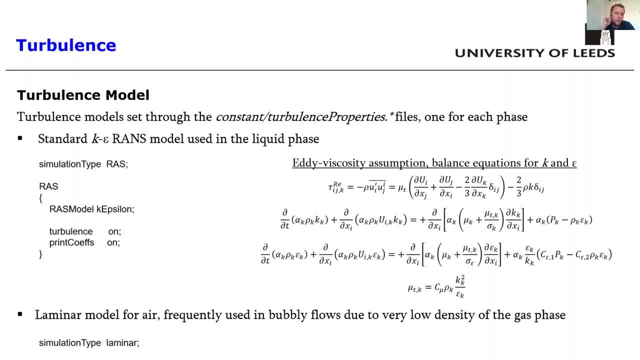 we solve one equation for the turbulence kinetic energy and one equation for the turbulence dissipation rate For the air. instead, we consider a laminar flow of air, and this is normally acceptable in bubbly flows because air has a much lower density with respect to the air flow. 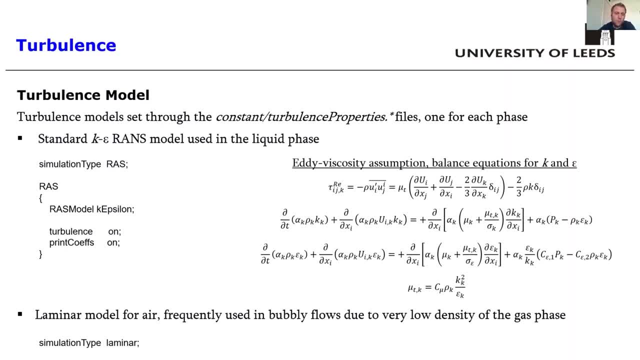 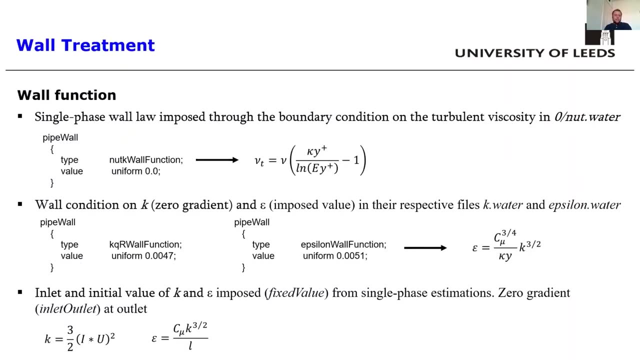 So the turbulence model is not suitable for the air phase and so it won't have so much effect. so it's actually absolutely fine to neglect a turbulence model for the air phase. Next, let's move to. the important thing is at this point, since we have defined the turbulence model, is: 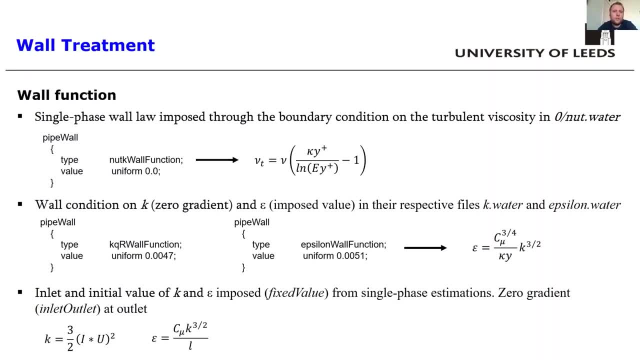 how we uh and we have a wall, which is quite important in this case, how we model the wall region and what wall treatment we use. In this case we use a wall function approach, so a high Reynolds wall treatment, and we use the single phase wall low at the wall and this is imposed using the. 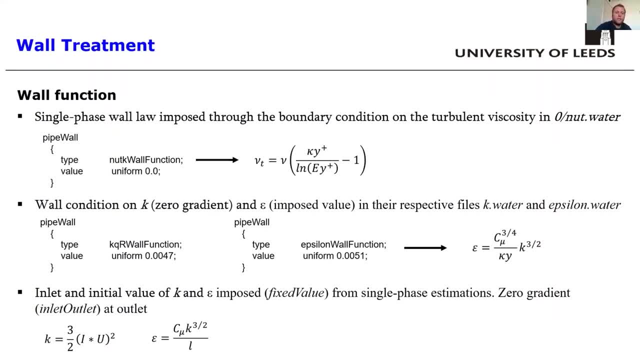 boundary condition for the turbulent viscosity. and you see, here at the wall we have imposed the wall function boundary condition and so the turbulent viscosity there is imposed to respect the law of the wall or following the law of the wall. At the wall we have a zero gradient condition for the turbulence kinetic energy, instead the turbulence. 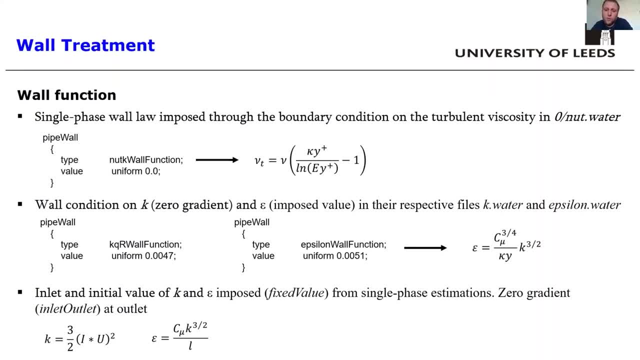 dissipation rate is imposed in this first cell near the wall, and those are again done using the pipe wall boundary condition in the file for the water turbulence, kinetic energy and epsilon. As you see there, for the pi, for the wall, for the k I use a QQR wall function. 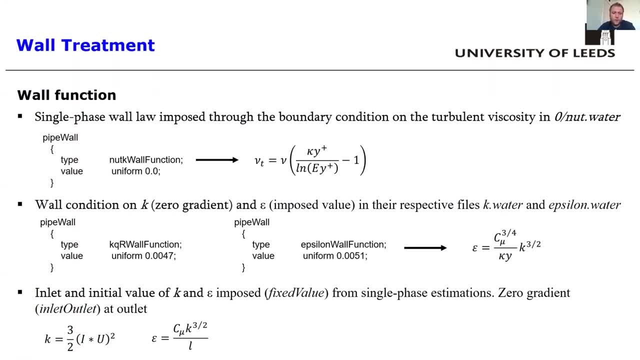 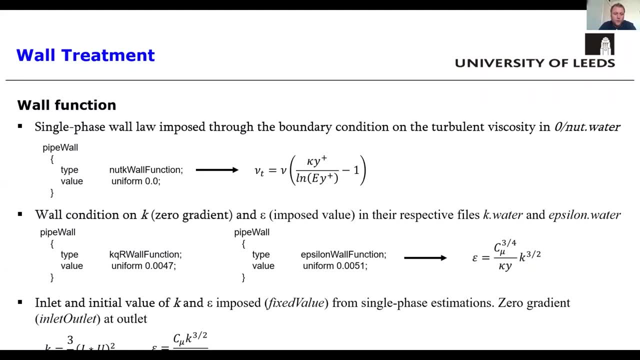 maybe now I will switch just for a moment to the files. For the turbulence kinetic energy the zero gradient is imposed using the wall function boundary condition, which is essentially for turbulence. kinetic energy imposes a zero gradient condition And instead for epsilon we use the epsilon wall function boundary condition that fixed the value on that last cell near. 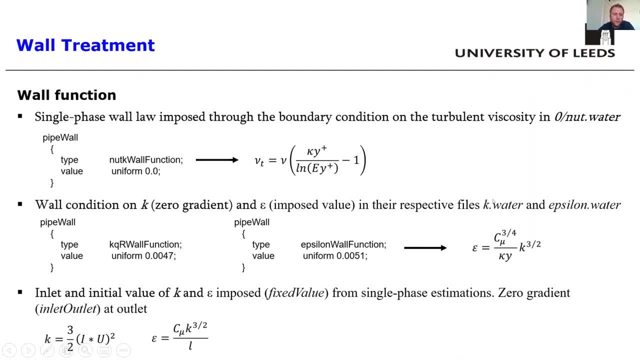 the wall to this value here prescribed by theory For inlet and initial condition on both k and turbulence dissipation rate. we use some single phase estimation to have a little bit of turbulence coming in the pipe and at the beginning of the simulation And you see the equations used for that calculation And we have zero gradient condition at the. 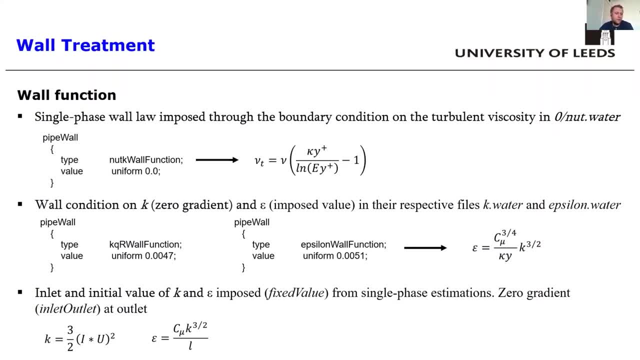 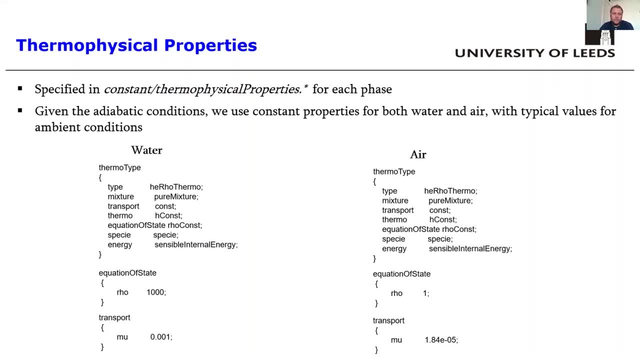 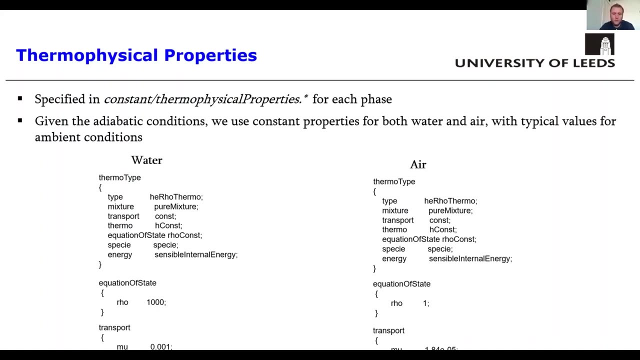 outlet And using the inlet outlet condition. The other things to set now we have cover more or less everything that is important in the zero folder. So initial and boundary condition: We have covered the turbulence models, Another thing we need to cover in setting up the cases. 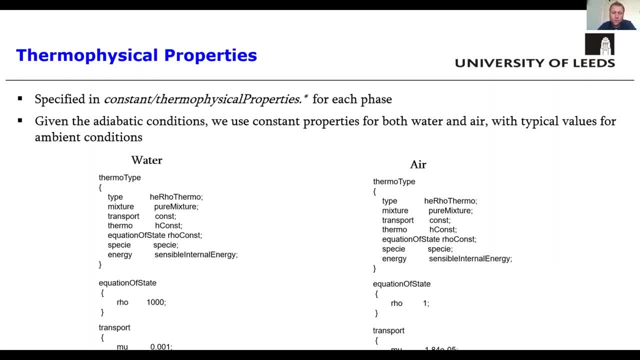 of course, the properties Of the two phases, which are again specified differently from air and water file for each, and a thermal physical properties file for each. There's not really a lot to say. It's a case with adiabatic conditions, So we use constant. 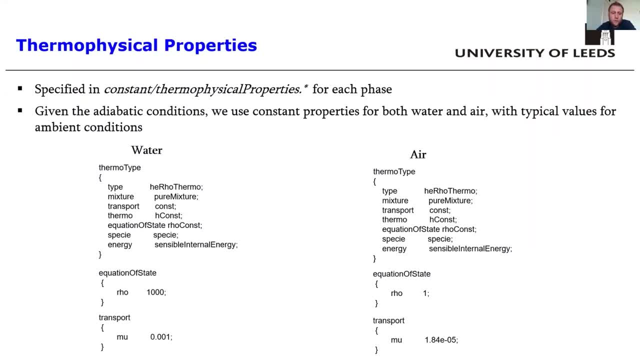 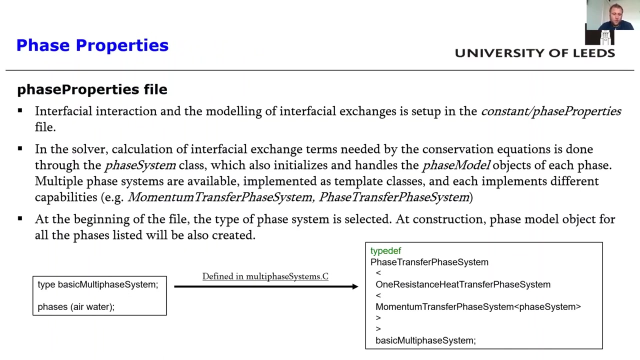 properties for both air and water and we use typical values that are valid for ambient conditions. So you see there that we have a constant density considered for both phases and that is acceptable for this case. Now, probably the most important files there is, you see that there is this phase property. 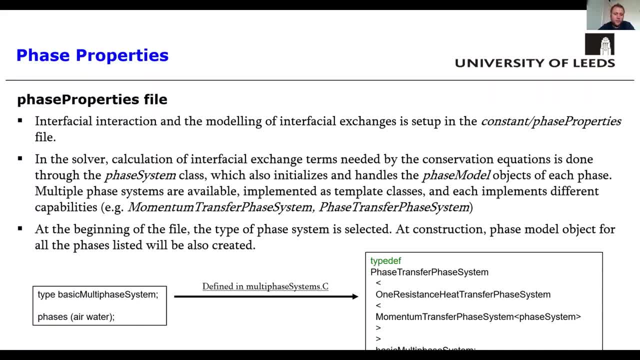 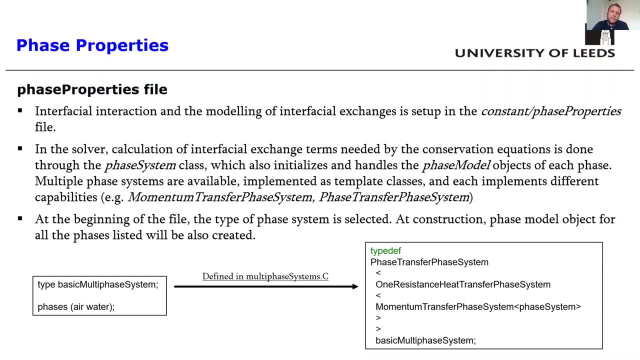 files. So we have set up everything, but we have not yet talked about what I mentioned at the beginning. So all the interaction Between the phases that is really key to correctly reproduce these bubbly flow, and all these interaction and all the interfacial exchanges is handled by the phase system model. 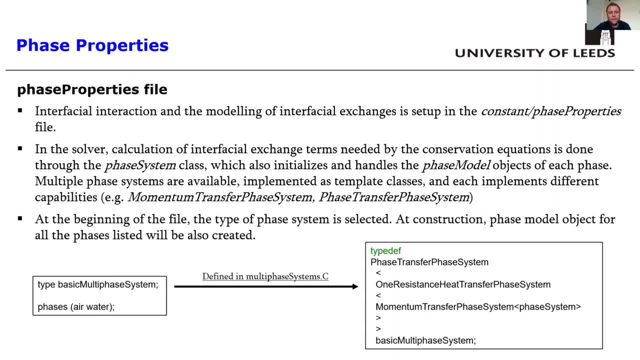 and which forces or heat transfer mechanisms to considered between the phases are declared in this phase properties file, Which is located in constant. Now The base class that handles all the interfacial interaction is the phase system class and order. then calculating the different terms, source terms for momentum interaction, energy. 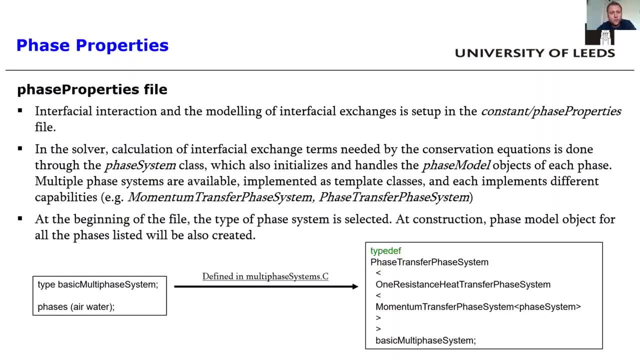 interaction that goes in the balance equations. that also initializes and handles the single phase models for each phase. Now there are different types of phase system implemented in this code and these are implemented as template classes so that they can be added step by step, Starting from the base class. 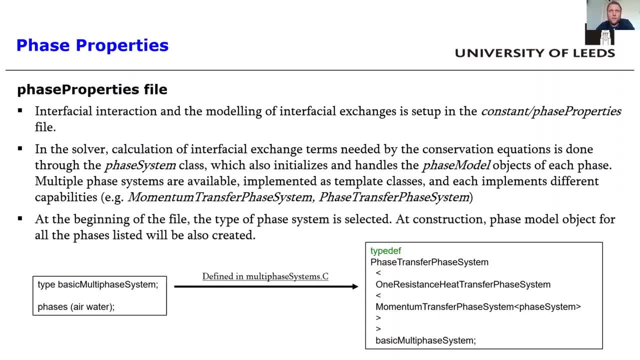 This is because each one of these phase system does a different things. So we have the momentum transfer phase system that implements the function needed to calculate the interfacial momentum interaction. Then we have the phase transfer phase system that does the same for mass transfer, and then 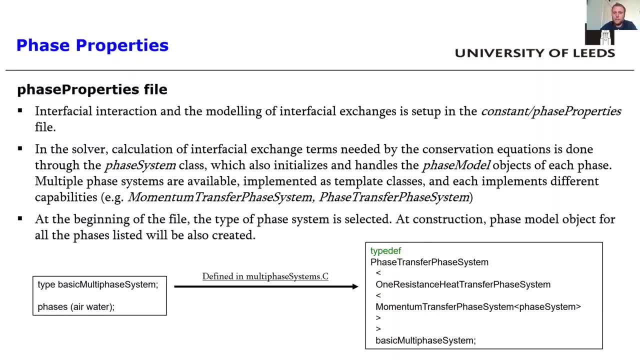 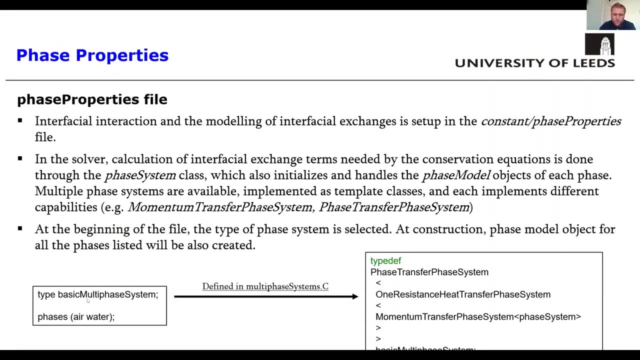 we have different heat transfer phase systems That does that in different ways for the for the heat transfer. So the type of multi-phase system we use is declared at the beginning of the file. Let's go in the file here Here at the beginning. first thing we declare is the type of phase system we want to use. 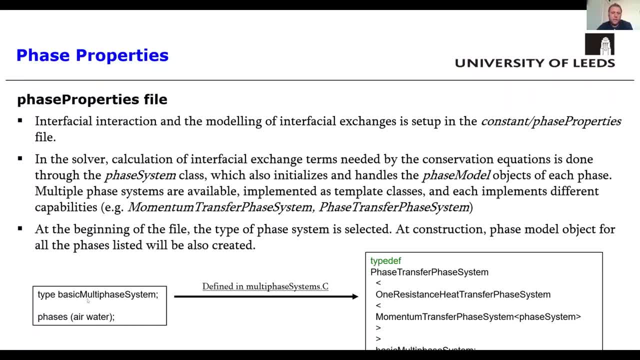 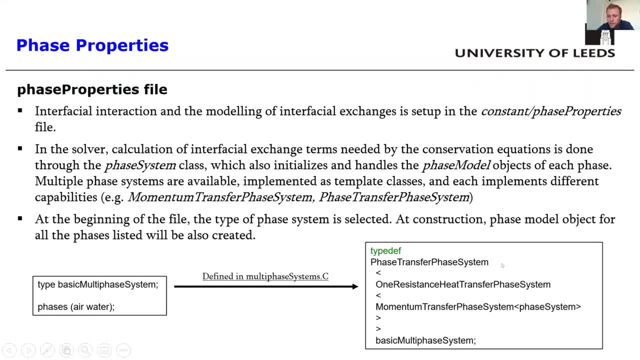 which is basic multi-phase system. in this case, What does mean that is defined in the multi-phase systems? So We have the c file and you see on the right its definition. So we have the momentum transfer, but also heat transfer activated and also mass transfer. 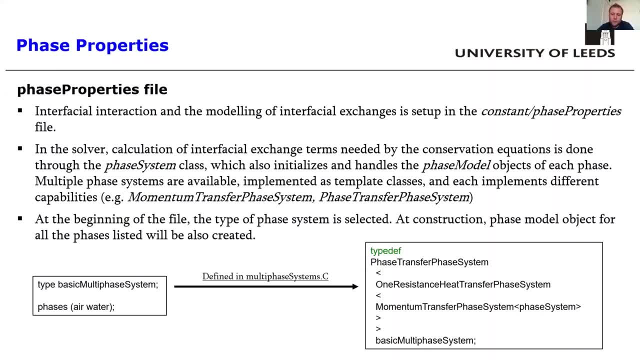 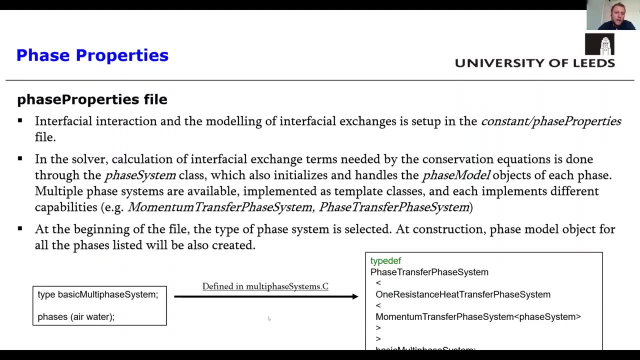 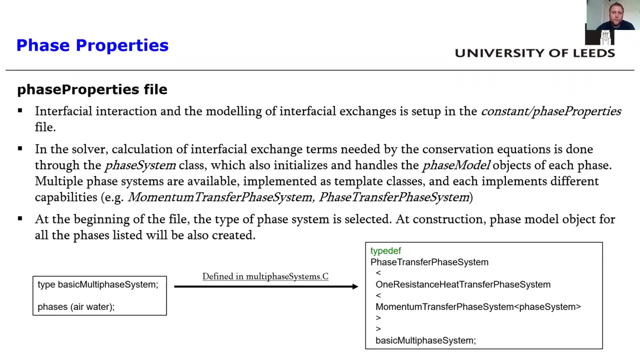 activated. We don't use those in this example, but that is the most basic phase system that is available. After that we declare the phases we want in our system, So two phases- air and water- And after that we need to declare the main properties of these two phases. 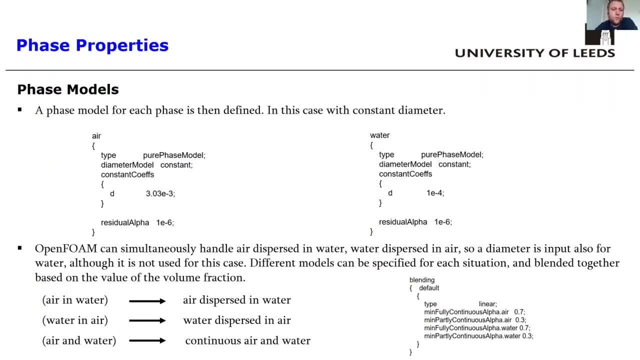 So we have a dictionary for each phase, one for air, one for water. They are declared as pure phase model and, as I mentioned, we can consider a constant diameter. so the diameter of the air is considered constant, is imposed constant, with the value equal at the experimental value. 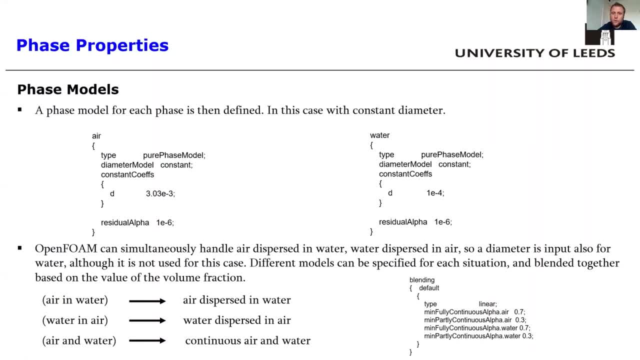 And as you see, there we have to impose a value of the diameter also for the water. Why is that? because for each case OpenFOAM is able to handle the entire range of volume fraction concentration. So we can go for air dispersed in water to at much higher gas volume fraction water dispersed in air. 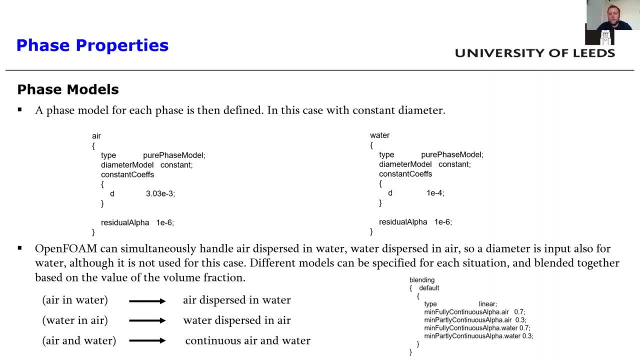 So if that happens, The value of the diameter stays the same, So we can go for air dispersed in water to at much higher gas volume fraction. water dispersed in air, Because that is considered, is that imposed for water. You want to happen in this case, but I just wanted to mention this as a additional functionality of the model. 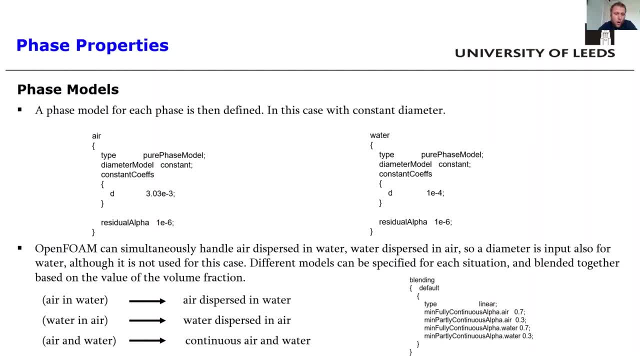 and in this way the motor can take into account different flow regimes that can happen in the flow and select the right, The right closure relation for the interfacial exchanges for each floor regime. How we do that by specifying different model based essentially on wording. So you see, on the bottom left. 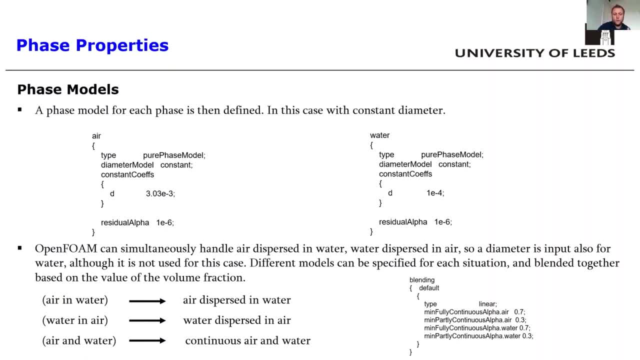 you have. air in water means air dispersed in water, So each model defined for air in water will be active when air is dispersed in water. Water in air means instead water droplets dispersed in air and instead air and water is in between, or can also mean two. 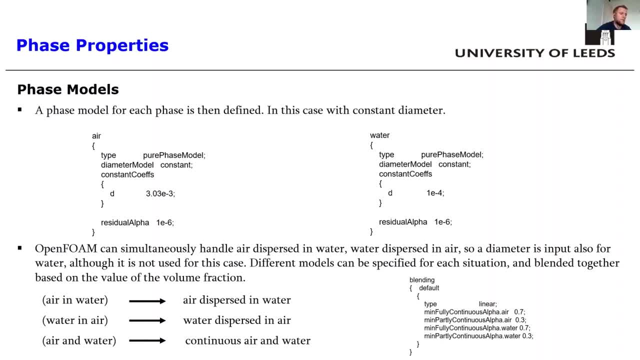 continuous gas and gas and liquid continuous, separated by a large interface. And now these are blended together by the blending dictionary, which means we define a sub-model, a drag model for each of these three and until the gas volume fraction is 0.3, from 0 to 0.3,. 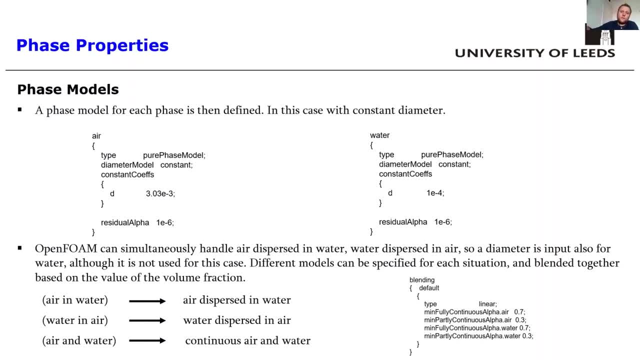 that case, is air dispersed in water Higher than 0.7,. 0.3. is air dispersed in water Higher than 0.7. is air dispersed in water Higher than 0.7. is air dispersed in water Higher than 0.7,. 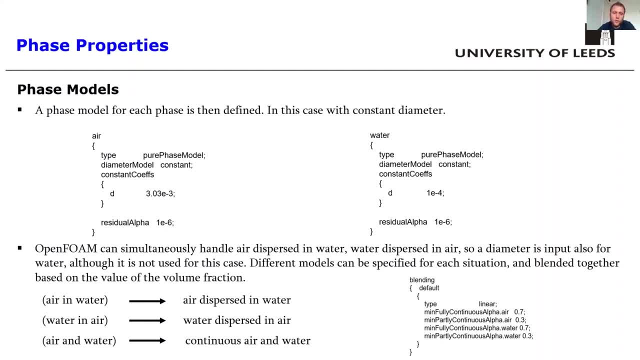 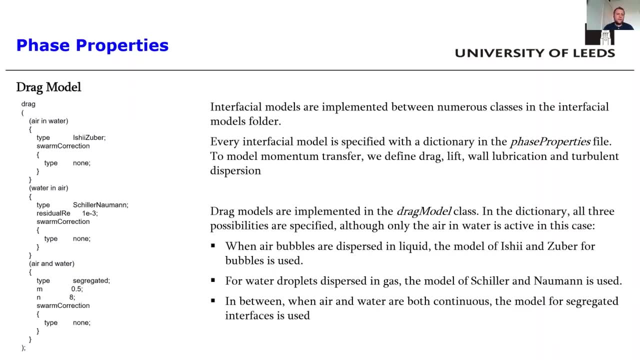 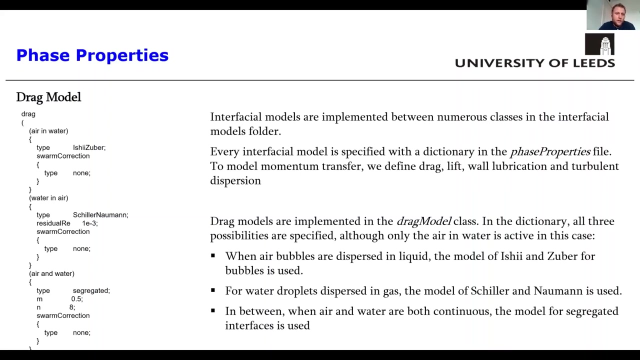 0.7 is water dispersed in air And in between we have a blending between the three different models. And here I've left an example, also in the file you see there, for the drag. Again, it's not needed in this case. If you define only air and water, that would be fine enough. 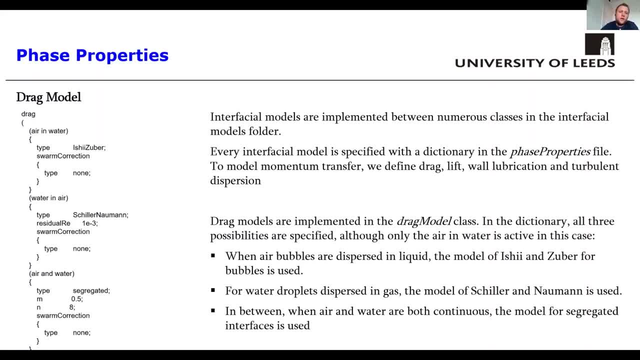 I've left it there just to show it works. So for air dispersed in water we use the Ischian-Zuber drag correlation. If the flow switches to water dispersed in air, the Schiller and Neumann correlation will be used In between the segregated model for large interfaces. 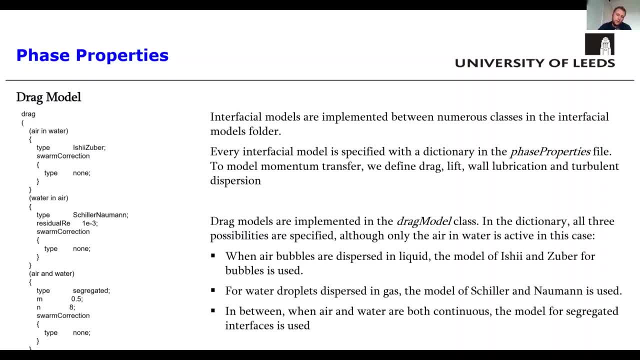 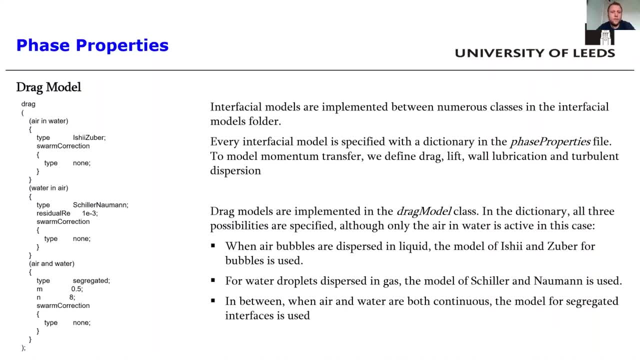 is used And essentially there is also how we define each sub-model with a dictionary. All these interfacial models are implemented between numerous classes in the interfacial model folder, in the React Angular folder, main folder, And every interfacial model is 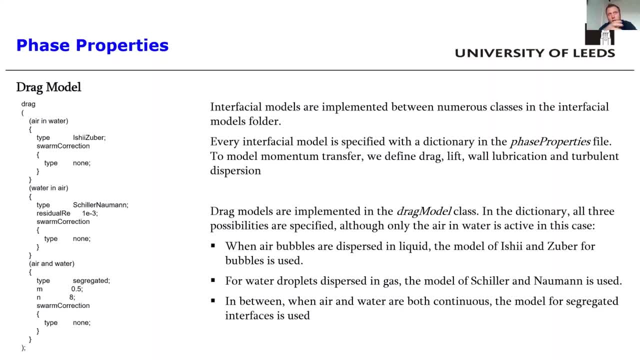 specified as a class. So in this case we have the drag model class which handles the drag model. So there are many models available. You can have a look at the flows if you go in the interfacial models folder. In this case we use the Ischian-Zuber. 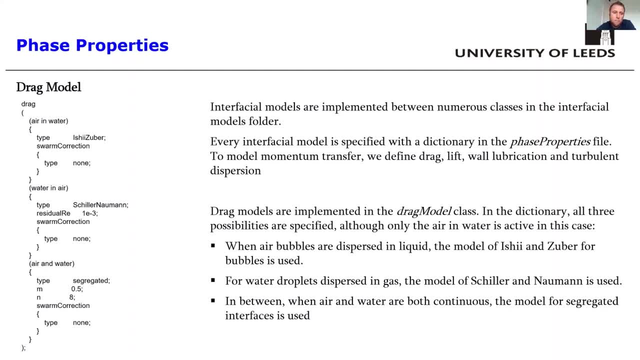 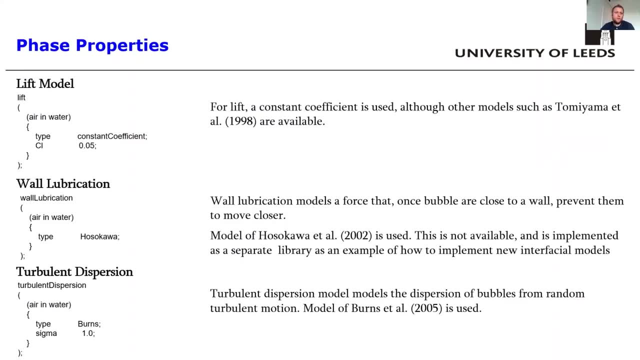 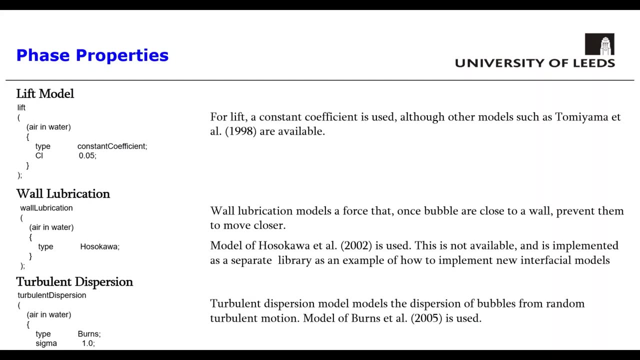 correlation, which is quite frequently used for bubbly flows And instead for the other forces. as Let's go back, Marco, sorry for interrupting. Are you sharing also the terminal or not, Because we can only see the presentation? Oh yeah, sorry, I didn't realize that. I thought I was switching between the terminal. 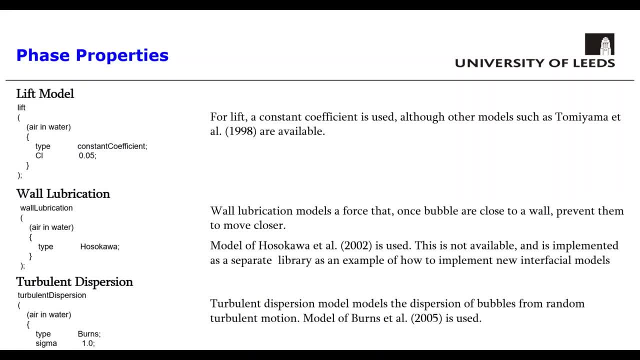 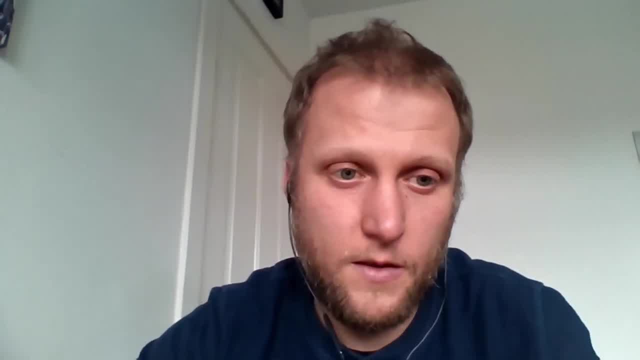 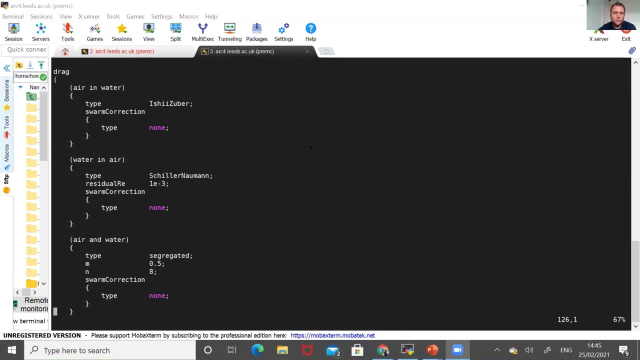 and the No problem. So how do I do that? Let me, I think you need to. Can you see the terminal now? Yes, now we can. Oh, sorry, because I probably shared directly the presentation. No problem, I think. well, most of the thing that you explained was also in your presentation. 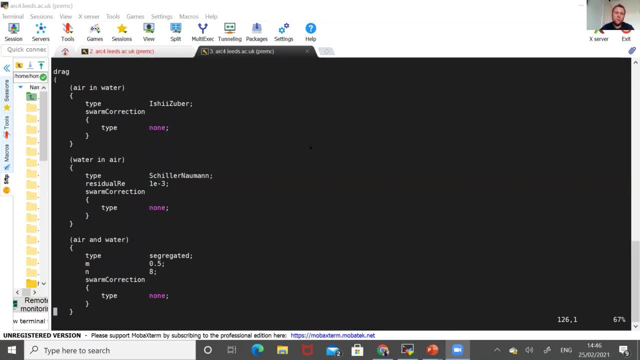 so, Yes, yes, that's true. I hope it was clear then. Okay, so now you can see the drag dictionary with all the model Great, Sorry for the interruption. No, no, actually. thank you very much. I should have noticed before And then later on below. 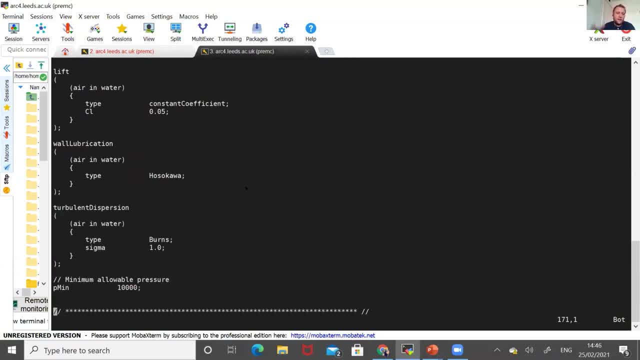 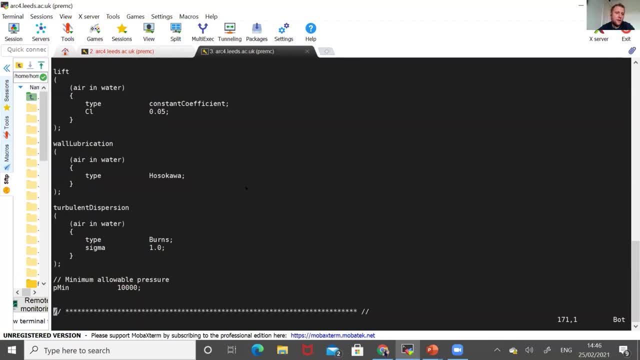 How do you feel, Drinf楚i? I think we have a great DENNIS here. Yeah, Hello, Hello there. Conference. Can you be faster in glucose by tonight? I don't know if it can be beetle, Is this for free? 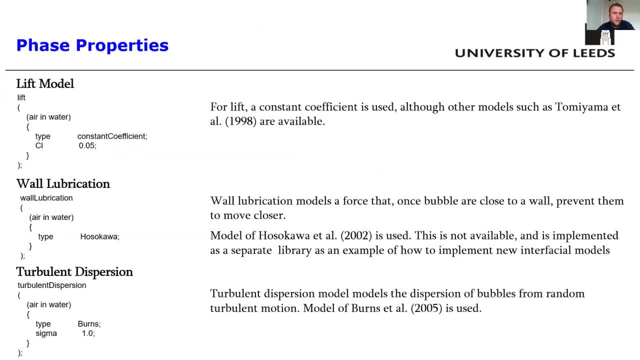 Oh look, sorry. Okay, Good, No problem. So how do you feel? I hope it will be speakable. Yeah, But I do have a slight problem with high temperatures. Yeah, Against the enters. Yes, I think that you know. these standardonents will not not only allowing you to be available. 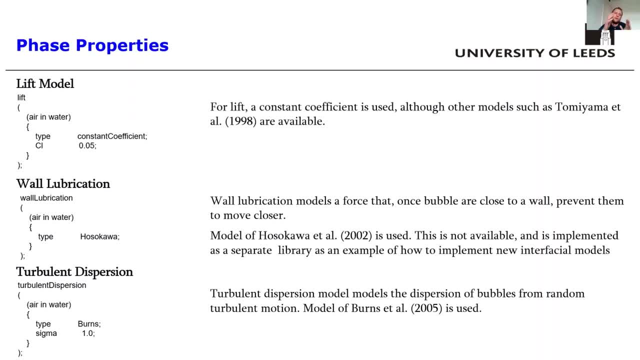 nine stored costs, but you have to stay alive for four months, whether you have to catch a cold or something like that. Yeah, Yeah, bubbles lift will push the bubbles towards the wall and the wall- lubrication- is a force that acts in the region, in the very narrow region, and prevents the bubble to move further towards. 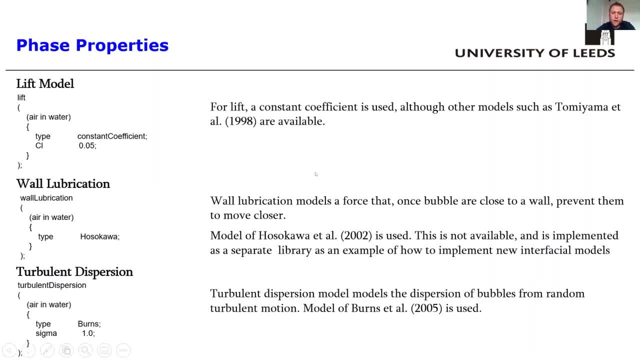 the wall. This is implemented using the Ozokawa model, which instead is not available in OpenFOAM, but I wanted to use this because I've provided this as an additional library and this is uploaded also in the Dropbox folder that you can use, and I wanted just to provide that as an example of 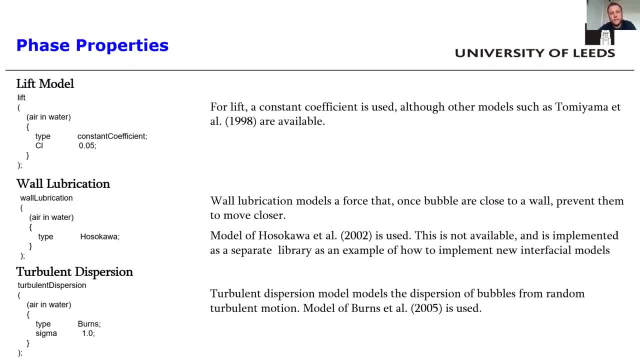 how to add an additional interfaction model that is not available in the model that is released. Then we had another force, that which is turbulent dispersion. that essentially models the effect of turbulence on the bubble. Turbulence will randomly make those bubbles and this effect is taken into account. 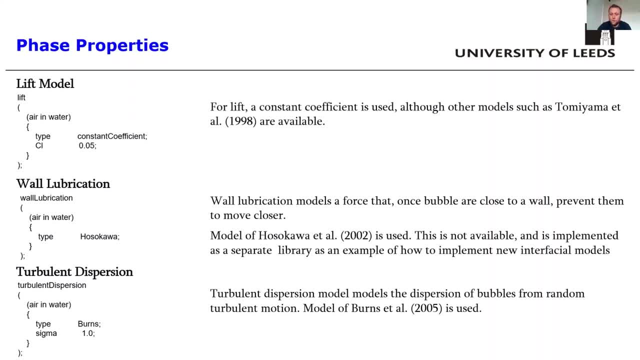 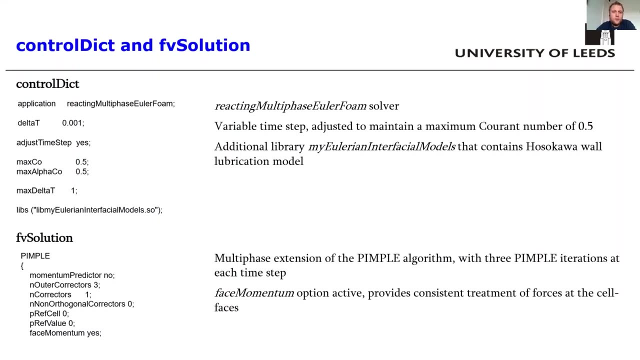 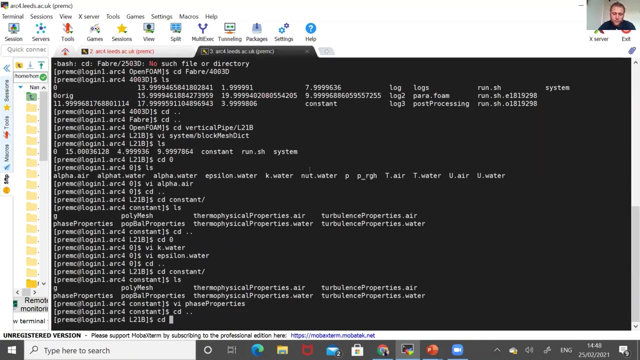 by the turbulence dispersion force and we select the model of Barnes. Yeah that, those are essentially all the forces we consider at the interface. and let's say a few words on the numerics and on the solution controls in our system folders. More or less the case is standard OpenFOAM. so we have 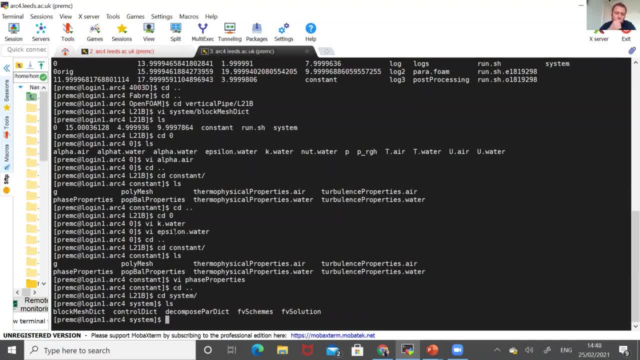 every scheme, every solution, control dict. we have the block mesh, which I talked I had shown before, but actually I didn't, and also we have the decomposed power dictionary that is needed if you want to run this simulation in parallel. Main things to say it's: 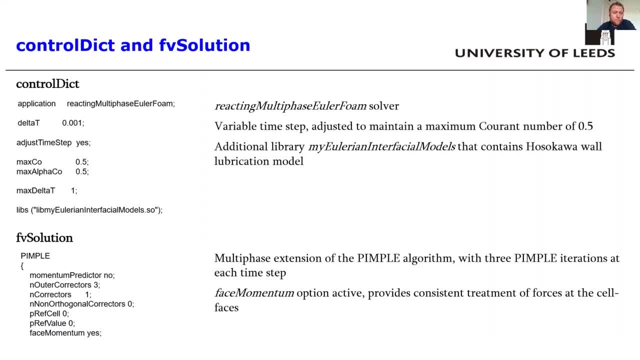 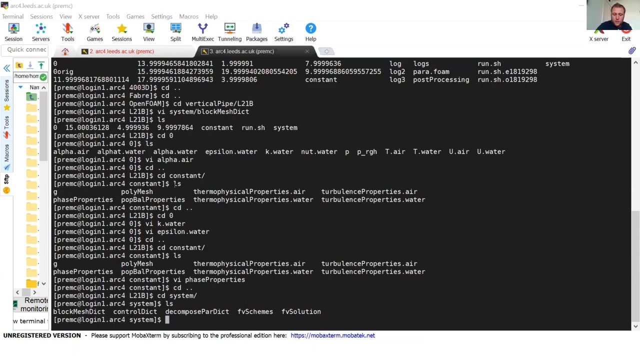 that we need to use a current number which is not too high. so the timestep is adjusted to maintain accurate number, not higher than 0.5. and also here you see that the additional library is added to. I'll show you also in the original file you see that this is above zero, so it's more or less similar to the existing. 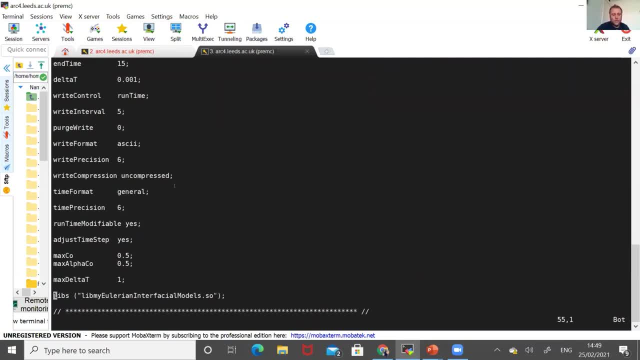 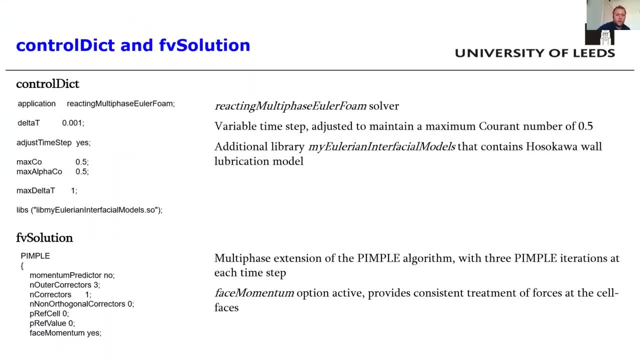 example library which contains the additional wall model, is added to the control dict file. For this solution, we use a pimple algorithm and we do three iterations of the algorithm, and the other things I want to talk about is this phase momentum option, which is a slightly 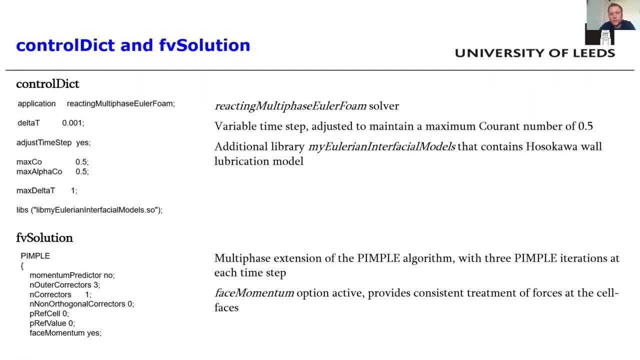 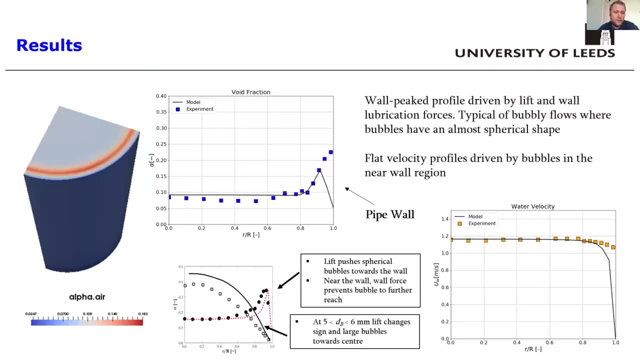 different formulation of the balance equation that provide a constant treatment of the forces at the cell phases and is is known to have some benefit to some in some particular conditions. Now let's have a look at some results, just briefly. This is a 3D image of the pipe. you see that. 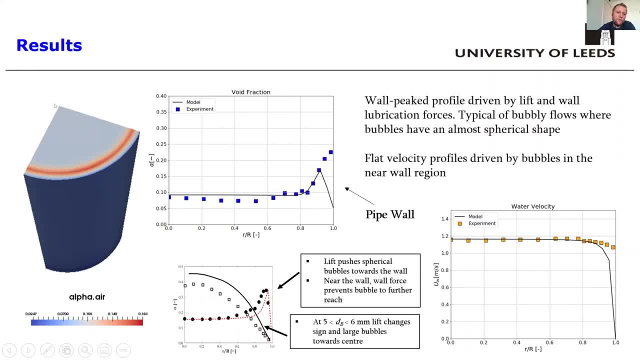 this is the volume fraction. you have an almost constant volume fraction in the center of the pipe, then a peak at the wall and a decrease towards the wall again, which is a common feature of these bubbly flows. You see that we don't predict perfectly well the experiment where. 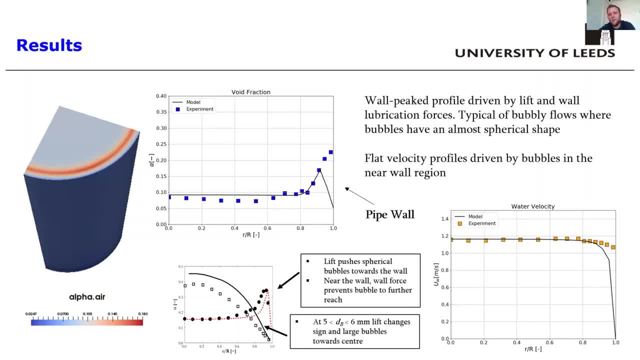 we predict that peak. That peak is not really really evident in this experiment, but I've provided some more results here for another case, And that's: the common features of bubbly flows is that peak at the wall for bubbles that have a near spherical shape, For larger bubbles, as I 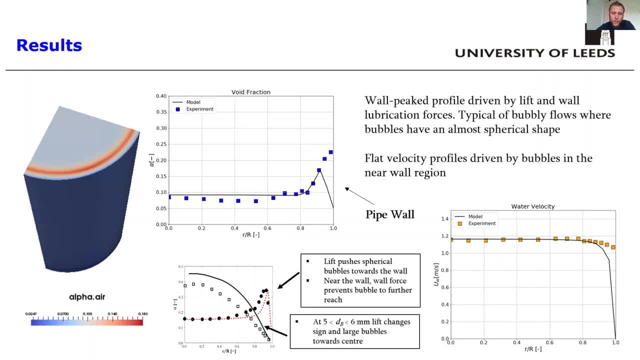 mentioned the lift for change sign. those bubbles are pushed to the center and you end up with this void profile that peaks in the center of the pipe. And I've shown also the velocity profile compared against the experiment, the water velocity, and you see how. 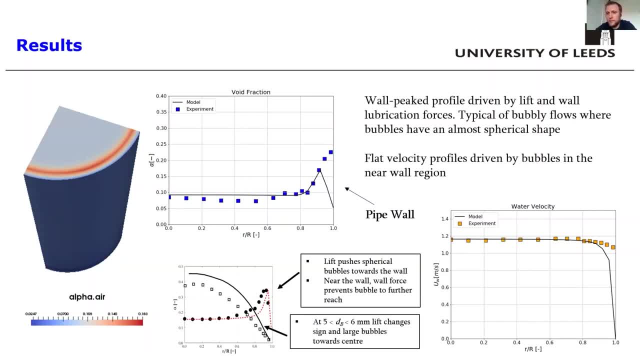 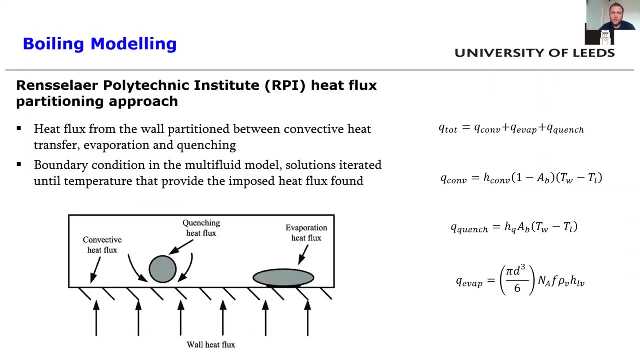 the effect of the bubble is to really flatten the that velocity profile with respect to a single phase flow. Now, this case, as I mentioned, is available in Dropbox and I think I'm running a bit late on time, so I will immediately go to. 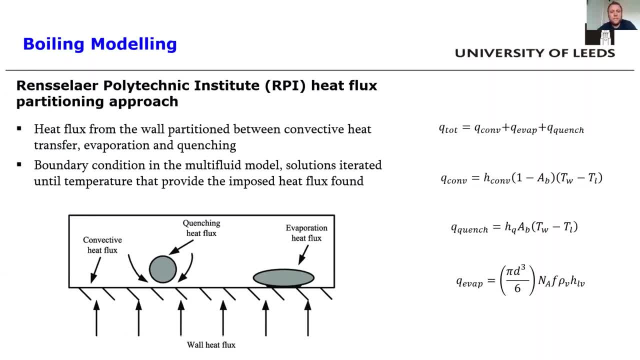 the next, which is, instead of boiling flow cases, more or less the same as before, but with the addition of a boiling model. So we have heat flux at the wall and this heat flux generates some boiling at that wall with the generation of bubbles, and this boiling is modeled using 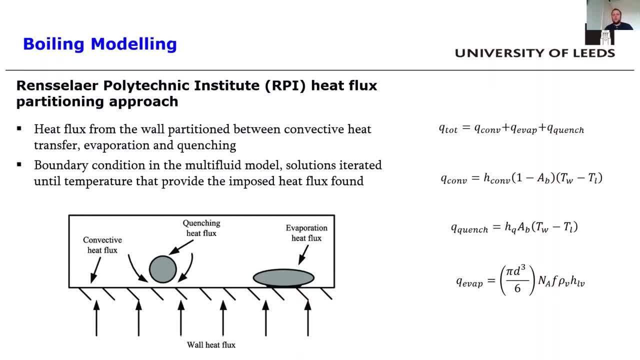 the heat flux partitioning approach. So we subdivide that heat in some contribution from single phase convection, some contribution from quenching and some contribution from evaporation. So they've taken away the production of bubbles that then detach and join the main flow. 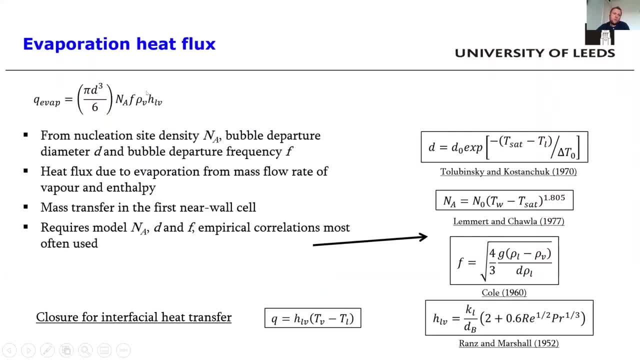 I want to focus on the evaporation, how the evaporation heat flux is modeled, because it's the main and the most important thing in this kind of model. So it is essentially modeled from the nucleation site density, so it's the number of nucleation sites on the wall that are active. 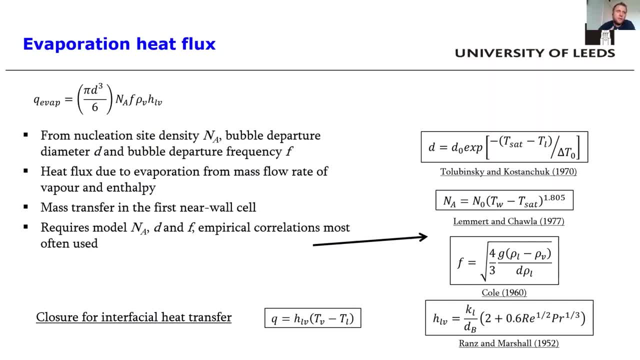 and generate bubbles. the bubble departure diameter- so how big is the bubble when it detaches from the wall. and the bubble departure frequency, which is how frequently bubbles detach from the wall. The essential product of those three plus the bubble volume is essentially a heat flux due to a mass flow rate of bubbles and multiplied. 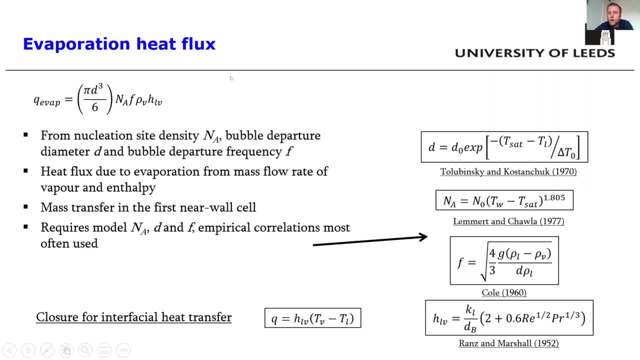 to their enthalpy of evaporation. All the mass transfer is in the first near-wall cell and this is always to take into account, that, because that makes the numerics quite challenging, And of course for the three terms that I mentioned, we need specific submodels. 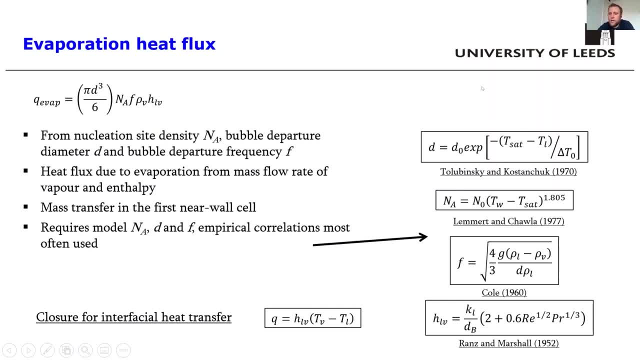 and I've put here some of the correlation that can be found in literature for departure diameter, nucleation site density and bubble departure frequency, and these are the models that are available in open format that I've used in this tutorial. Also, when bubble detaches, they join. 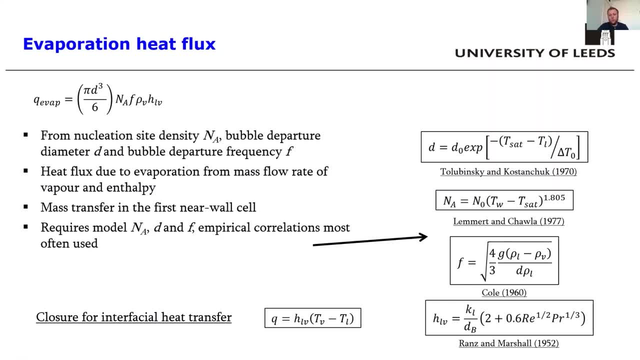 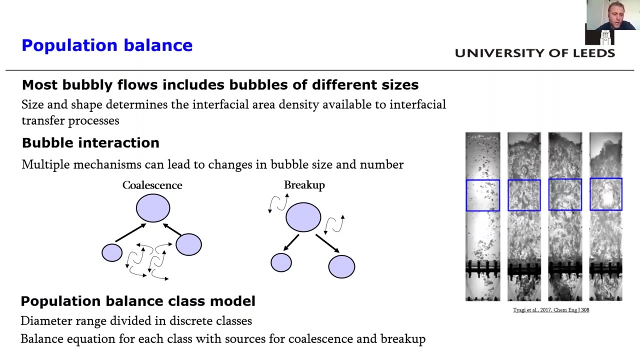 the liquid and exchange heat with the liquid. so we need to model also this heat transfer and this is done with an additional model for interfacial heat transfer. that is again closed, using an empirical correlation. An additional thing: before we have considered a constant bubble diameter. in this case bubble detaches from the wall. 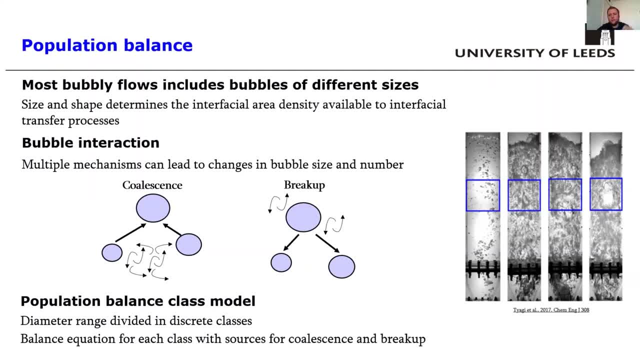 are very small and then they tend to grow up in the liquid phase because of interaction with other bubbles and so mainly coalescence. so bubbles collide with each other and coalesce and become bigger. Also the opposite can happen, mainly due to turbulence. so a large bubble can 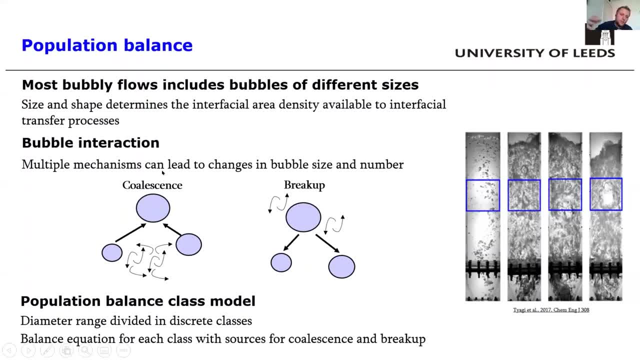 break up and divide in two. For this large change in bubble diameter in the flow we need to include also a population balance model and we use the population model balance models, the class population balance models available in open form, that subdivide the bubble diameter range into discrete classes and calculates, solves an. 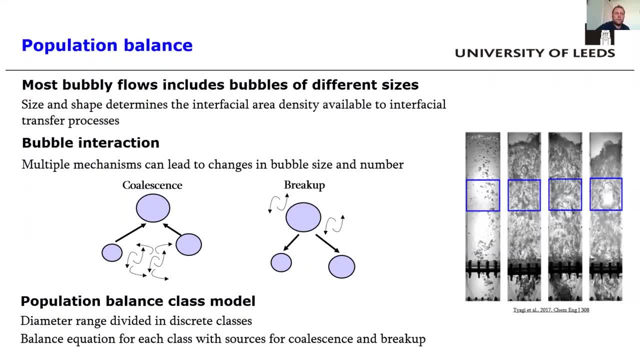 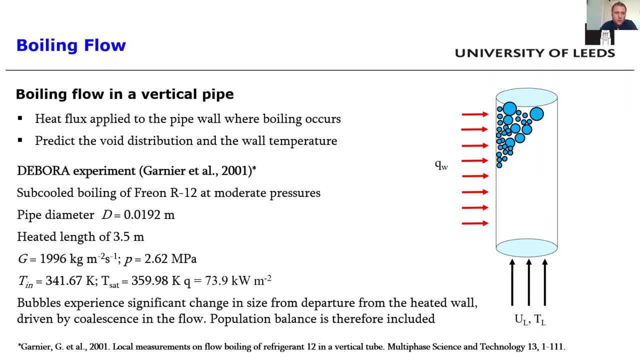 equation for each class and calculates the exchanges between the classes due to coalescence and breakup, And specific models for coalescence and breakup that are also included. So in this case, again we have a bubble boiling flow, again a vertical pipe with a liquid flow. 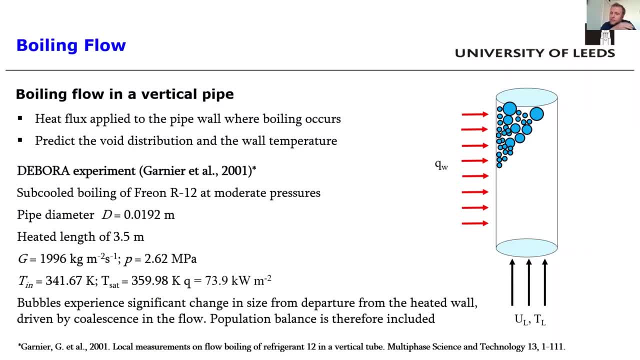 and this time single phase liquid. at the inlet it fluxes at the wall at generation of bubble due to boiling. We modeled this Debora experiment again, which is available for the subcooled boiling or refrigerant 12 at moderate pressure. This essentially is done because at those 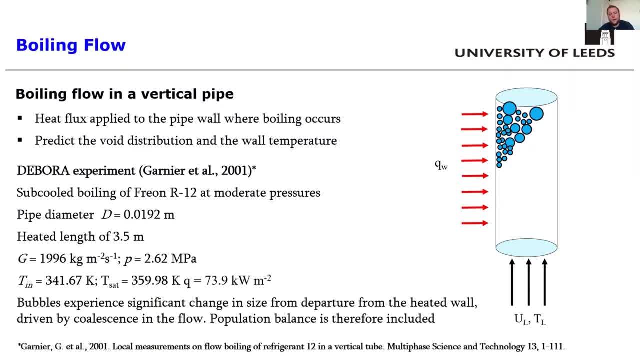 pressures. the refrigerant has the same non-dimensional number of water at much higher pressure at, in particular, the pressure of pressurized water nuclear reactor. but of course it's more convenient to run the experiment at the lower pressure. You see the the data we have and the setup, water at the inlet is subcooled, so is below saturation, and when? 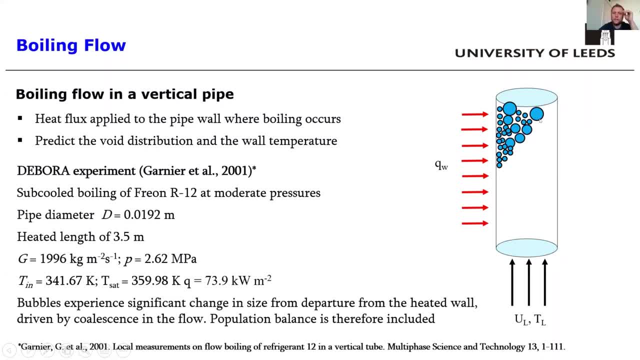 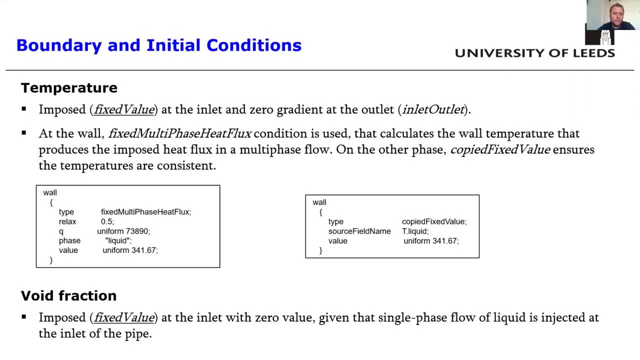 the temperature at the wall goes higher than saturation, then boiling starts in the pipe. Settings are more or less the same as before, but now we have temperature. so we have an unimposed fixed value of the temperature, of the temperature at the inlet, equal to the experiment and the zero gradient condition at 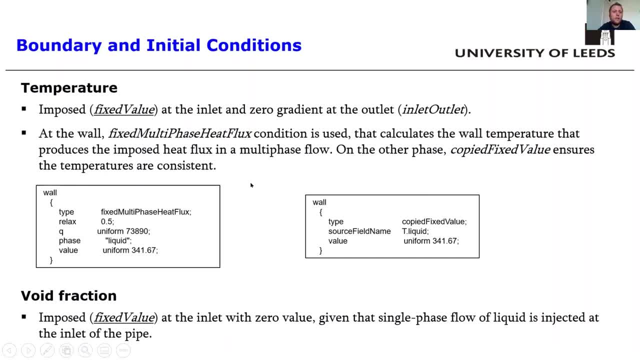 the outlet, again imposed with inlet outlet At the wall. the imposed heat flux is fixed using this fixed multi-phase heat flux condition, which essentially calculates the wall temperature that produces the imposed heat flux that we want in one phase, the liquid phase in this case. you see. 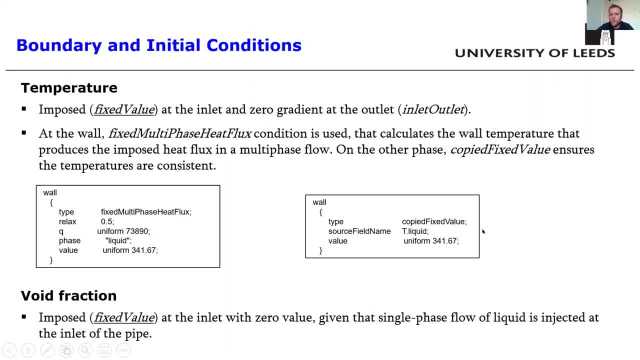 on the left, On the gas phase, we use the copied fixed value boundary condition, which essentially does the same thing but also ensures that the temperatures are consistent. Void fraction now is imposed again as a fixed value, but equal to zero at the inlet of the pipe, As I said, wall. 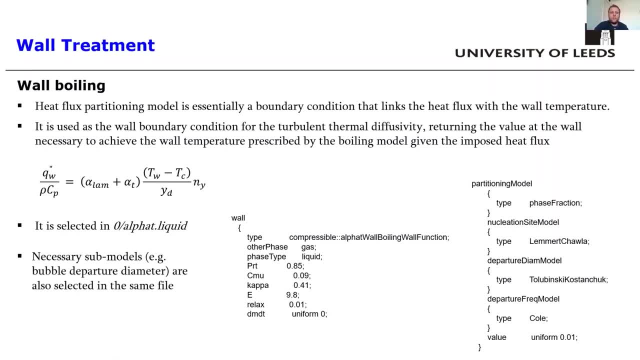 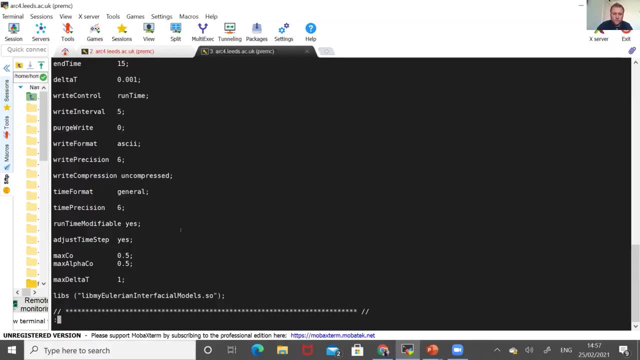 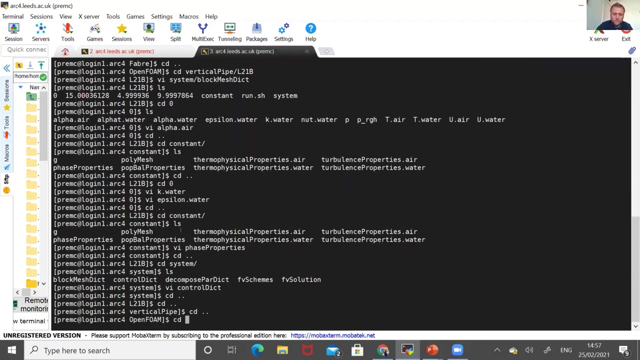 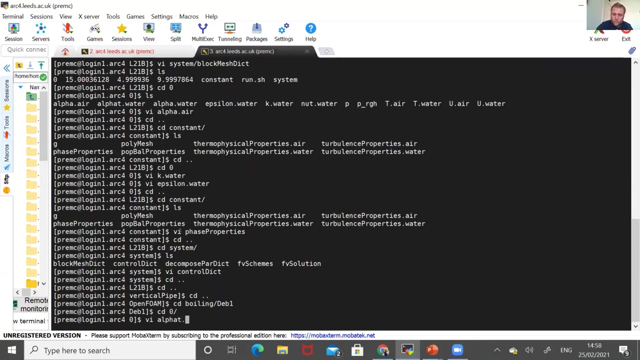 boiling is modeled using the heat flux partitioning approach where it is defined. This is defined in the thermal diffusivity wall boundary condition. so in this file here I can show that in the in the terminal. Okay, you see, we have the definition. this boundary condition is: 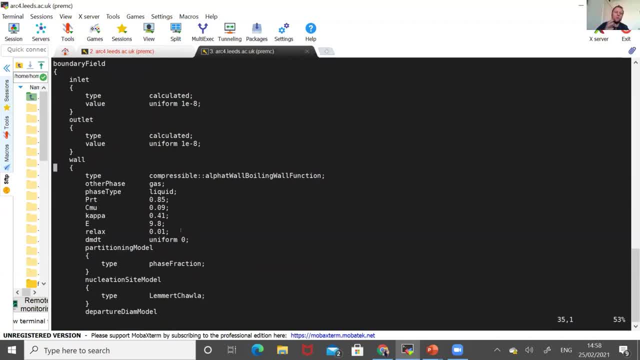 is essentially a wall function- visit flux partitioning model- that relates the wall temperature with the heat flux And it's activated by this wall function, The alpha T wall boiling wall function, again in the thermal diffusivity boundary condition of the liquid And you see the 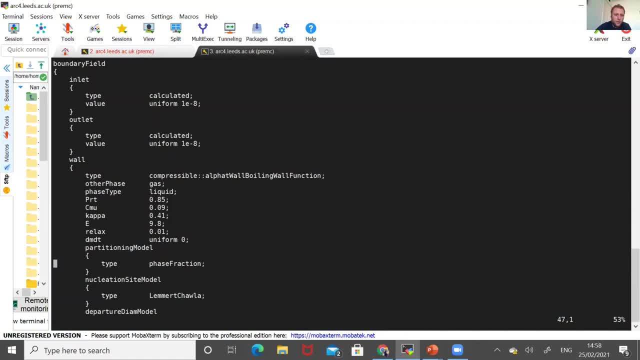 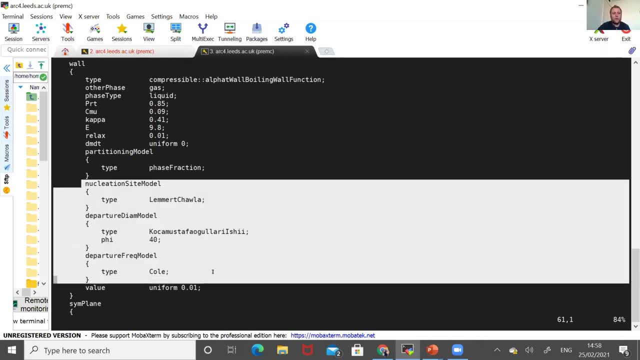 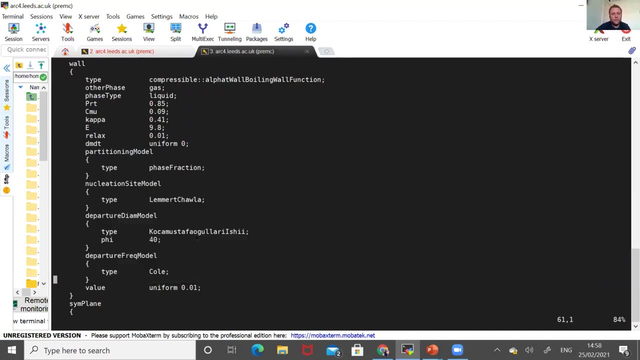 different parameters. there and also after it you can recognize the models that I mentioned before. So we have to define. with the model we defined we want to use for the nucleation site density, the departure diameter and the departure frequency, and you see that the model are defined there and those are. 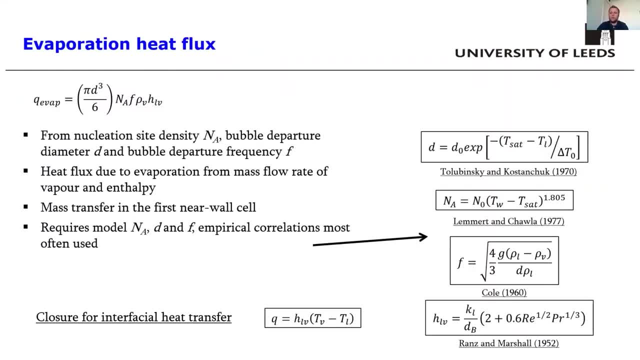 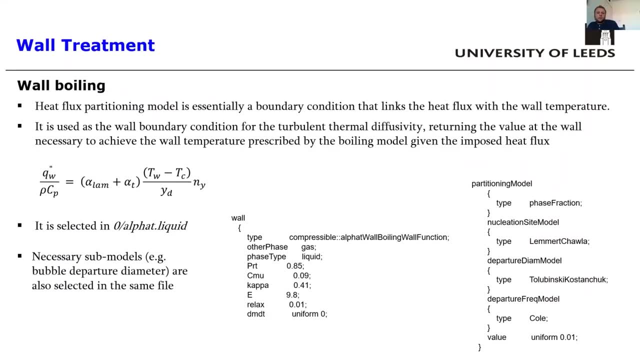 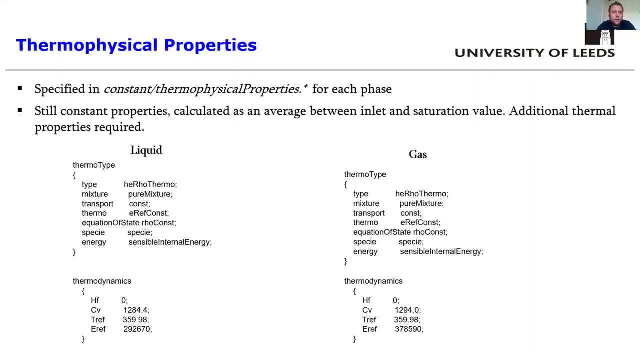 the model that i've shown here in the as they were derived by the authors of of those papers. then thermophysical property: again, we have considered constant properties here, and some are calculated as an average between inlet at saturation, for example the density. of course, other than density, now we need to define the specific heat and the um and the entropy of. 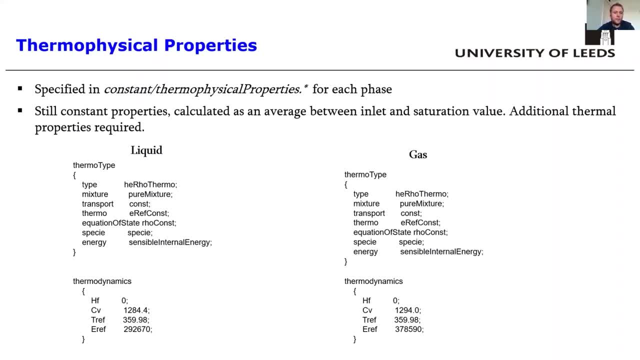 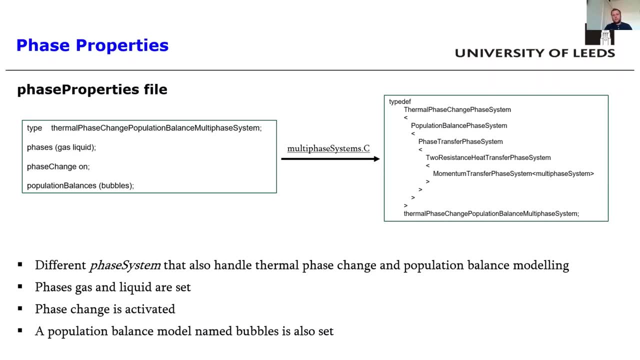 of the phases because of the phase change model that is now active. uh, we use now- uh, let's uh talk about the differences that there are in the phase property file again, where we define all our interfacial interaction. uh, we use the thermal phase change population balance. 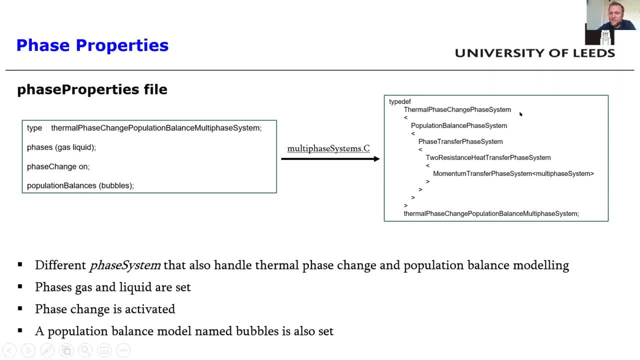 multi-phase system uh quite complex. it is defined here. on the right you see all the different phase systems that are used and active and, with respect to the previous one, those also has capabilities to uh to handle heat transfer and phase change and also a population balance model, and you see. 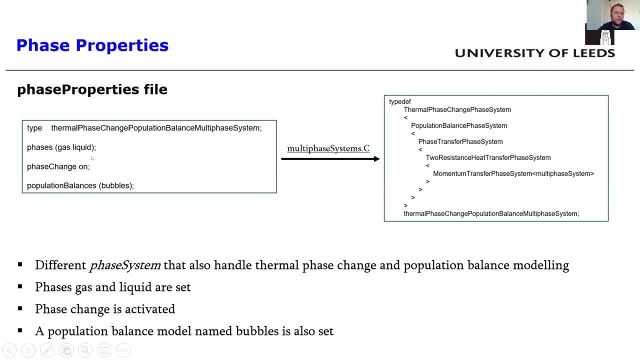 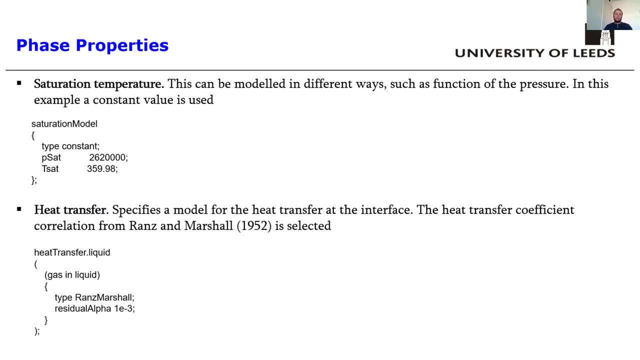 that again, after defining the phase system, we define the two phases. uh, sorry. we say that phase change, you know, is on and we also initialize our population balance. uh, on that, in addition to the model we have before, we have to define a model also for the saturation temperature. 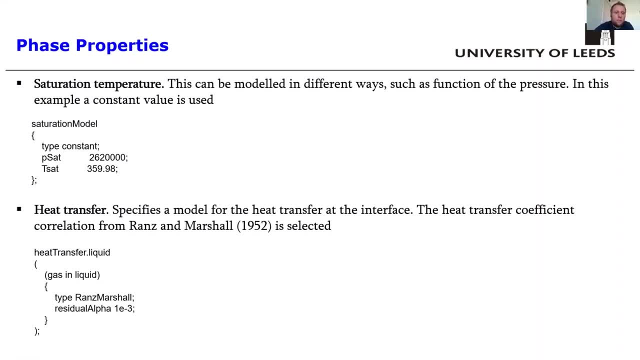 uh, different model can be used. can be um imposed as a function of pressure? in this case we have used a constant value of saturation at the reference pressure because essentially the change in pressure along the pipe is not that much, so it won't influence that much the value of the saturation temperature. 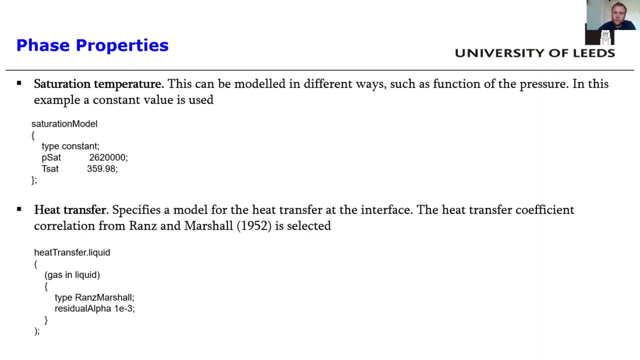 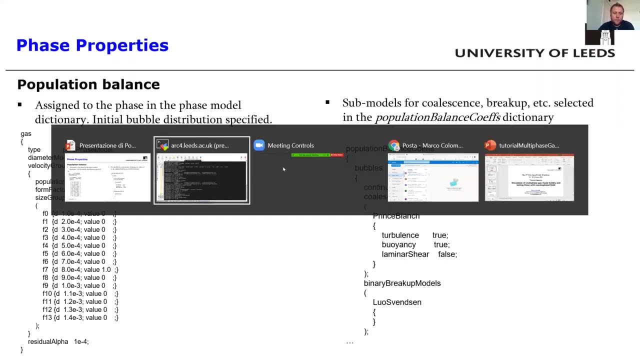 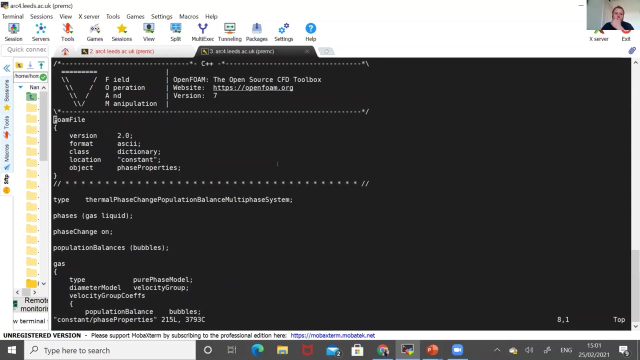 we also have to define the model for interfacial heat transfer. and you see that the runs and martial correlation is is declared there for the population balance. uh, i'll switch to the terminal. it's a bit more easier now. before we use the constant value, now we activate a population balance. you see here. 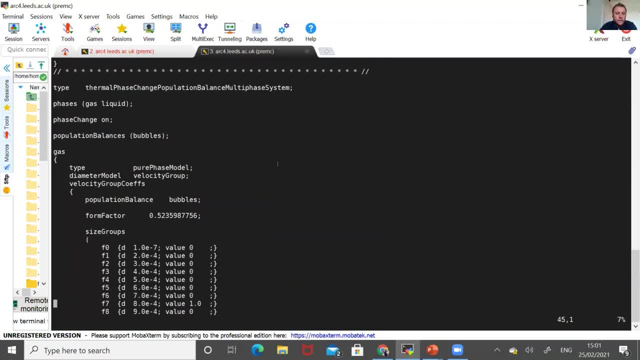 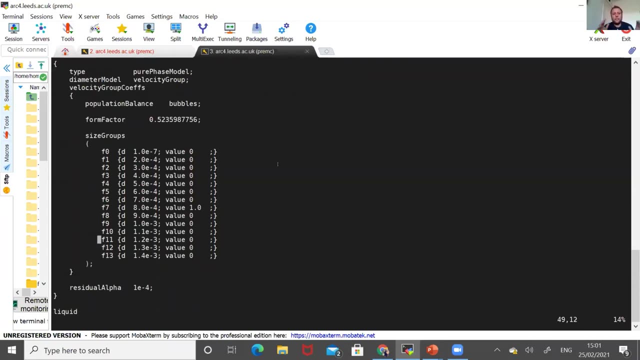 population balance bubbles and that you see here, that is defined for the gas phase. so the population balance, of course, is for the gas phase. uh, and you see that what we need to do is define size groups, which means that the bubble diameter range is subdivided into into those classes. 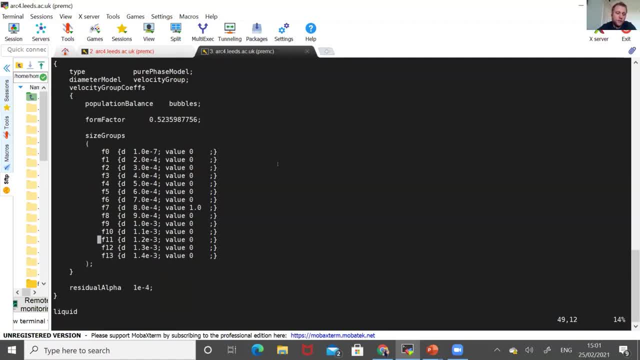 and those are the boundaries of the diameter between the different classes. and the other thing that is needed is this and this is population, but then the population balance coefficient, uh, that dictionary. instead we define the sub models that we want to be active. so you see here that 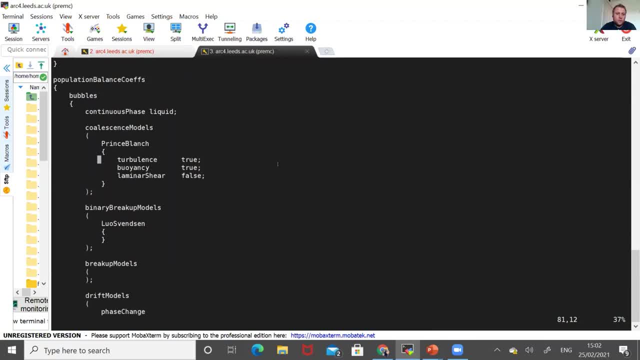 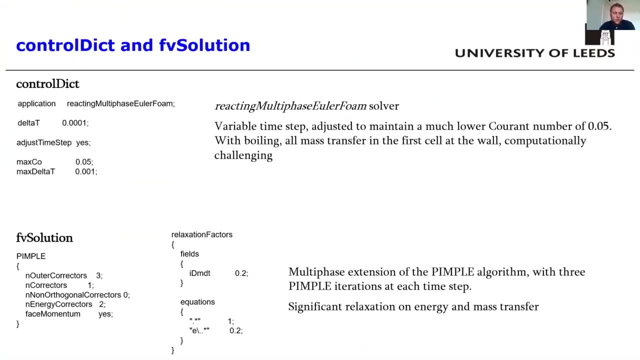 we have the coalescence model active using the Princeton-Blanche model and the breakup model is active using the Luo and Svensson model, and then we have other models active due to boiling and instead in the solvers, more or less, the settings are not that much different from before. the things to say is that this model. 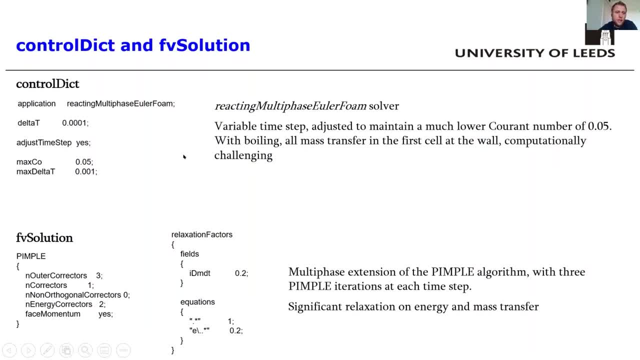 runs at very low current number. you see that here the maximum current number allowed is 0.05, which is quite low. This is because all the my transfer related to boiling happens in the first near-wall cell and that really makes the numerics quite challenging. Again, pin-pull loop is used with three correctors with three cycles. 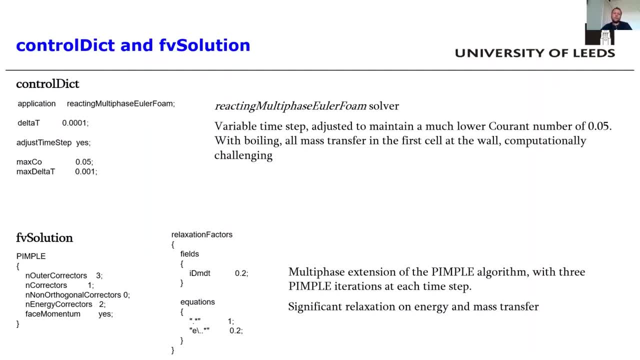 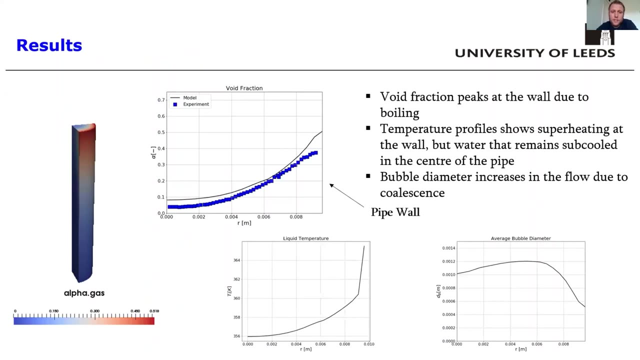 and you see that the relaxation factors also are quite low, in particular for the mass transfer, which is this one and what happened, and also the energy, and those are almost always needed when you're doing a boiling flow. Some results, as I did before. you see the volume fraction. 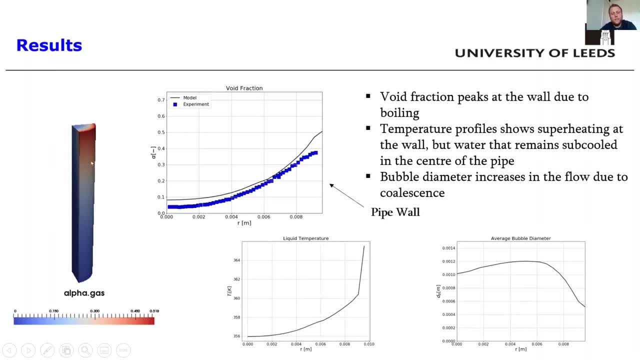 here that starts from zero at the bottom and then starts to boil here after half pipe and there is a significant boiling near the wall. You see the comparison against the experiment of the volume fraction quite good, not perfect, a bit too much void generated, but still good, You see. 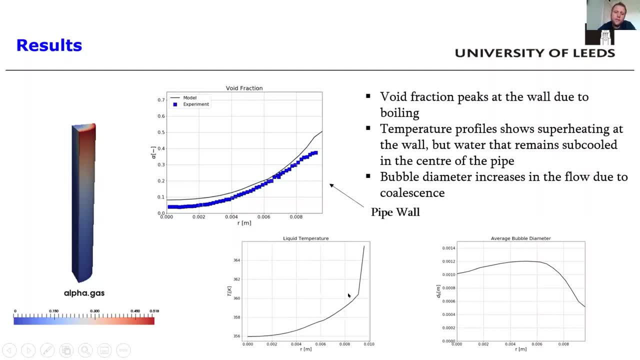 the wall temperature, the liquid temperature across the radius. here that goes from below saturation 356 in the center, so the liquid is still sub-cooled to over saturation, so boiling happening near the wall. and you see here also radial profile of the average bubble. 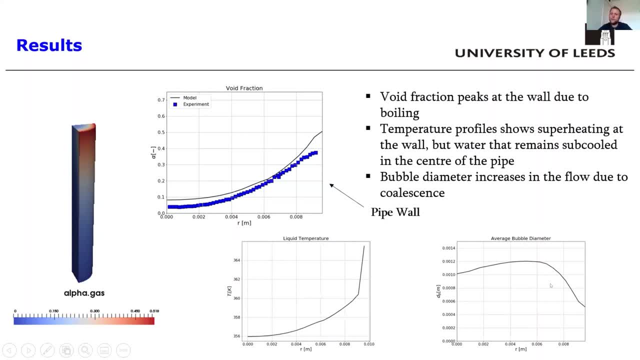 diameter. you see how bubbles are small at the wall and then increase in size because of coalescence in the center of the pipe. So I think- yeah, I think I'm just on time, a bit too long probably. sorry if I will cut. 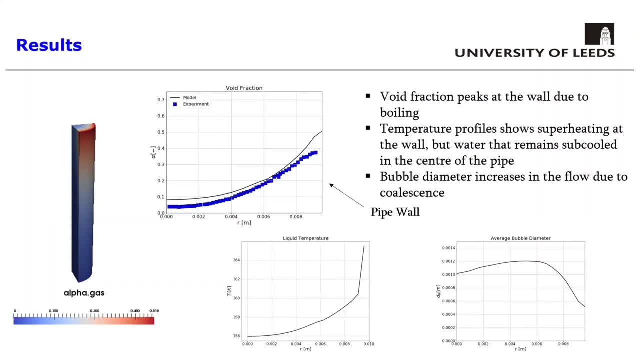 short the question. As I mentioned, the cases are uploaded in the Dropbox folder. One thing I want to say is they probably will take a bit longer to run that normal tutorial cases, but those settings, those those features or those settings of the model can be used also to model different cases. 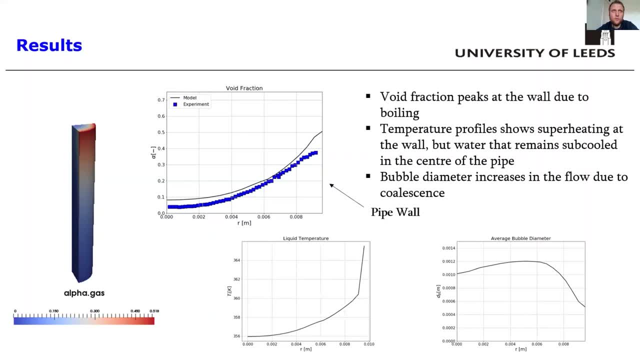 that are not a pipe, so that they can be used also for, for example, bubble column. same similar settings can be used, and they can. so therefore you can use those settings as a starting point for the other cases that you might be interested in. And thank you very much.